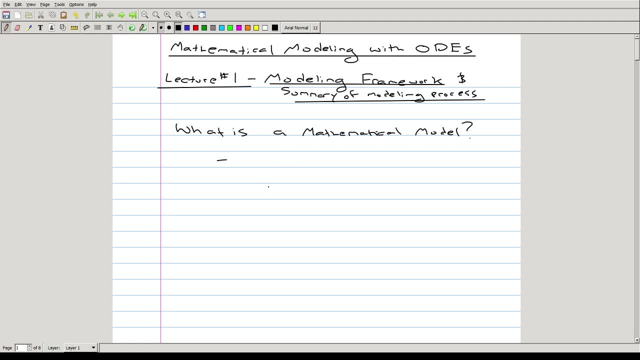 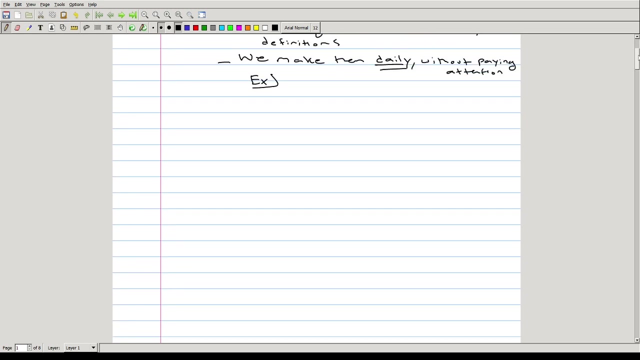 I guess I should start off by saying that this is a loaded question with many possible definitions. We make mathematical models daily without even thinking about it or without paying attention. And to give you a good example of this, think about one of the most basic questions that you might ask yourself. it's: how do I get downtown or how do I get to a place? 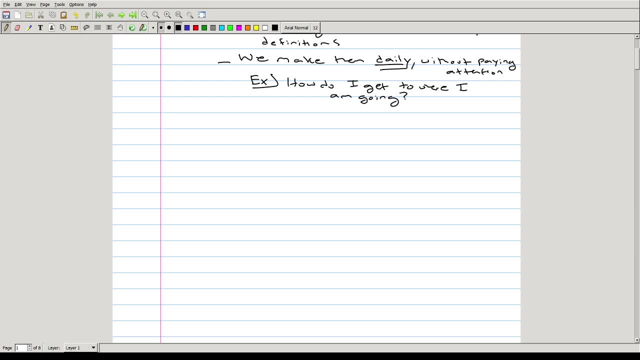 And there's many factors that you might consider, and you might not even realize that you're considering and weighing these factors against one another, but for one, the distance of where you're going is one of the factors that is going to factor into this decision, the money that you want to pay to get there. 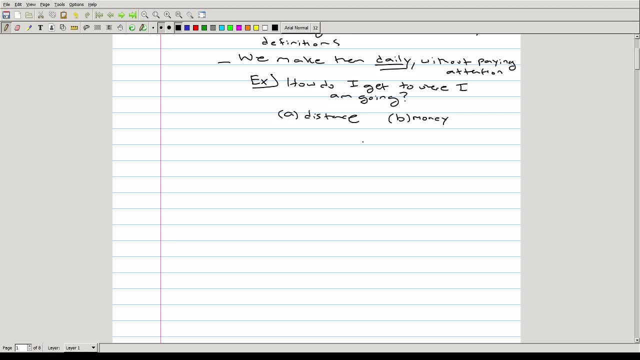 Whether you want to take the bus or ride a bike or drive a car. and this brings up another very important factor, which is time, or traversal time. How long do you want to take on the trip? Do you want to walk? Take a very long time, but if it's a short distance, you can walk in no time at all. 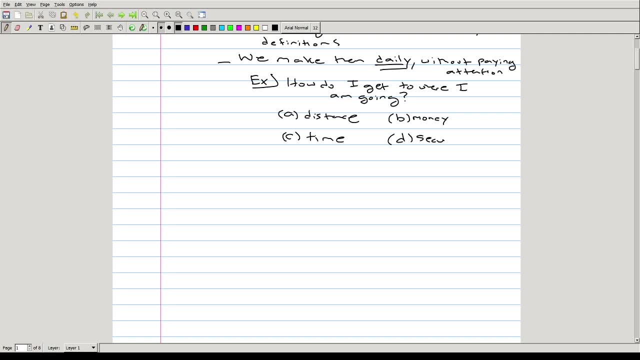 Another consideration that you might make is security. How do you want to get there? Do you bring money with you? Are you carrying money on you or anything valuable on you? And then this also brings up- you know, all these are kind of related to one another- but the means of transportation. 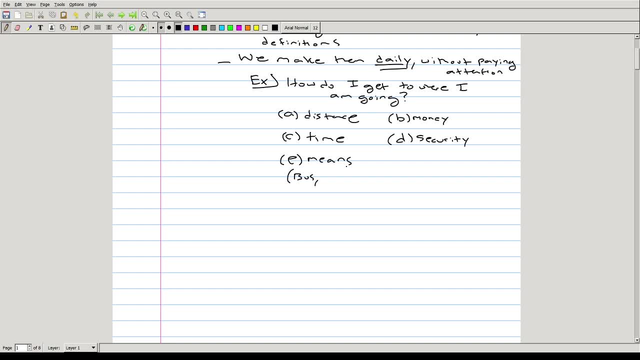 So, are you taking the bus? Are you going to order an Uber? Are you going to bike? Another factor, That is: you know your mood. Are you rushing? It's kind of related to time and distance. Are you rushing to get somewhere? Are you having kind of a leisurely stroll? 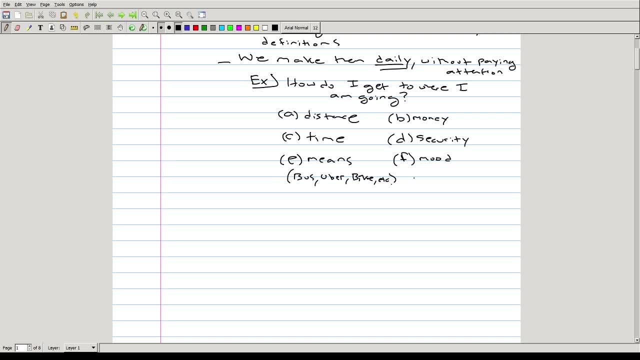 But you know, there are many other examples and there are also, in this example, many other factors that you might want to consider. but there's one simple example of how we create a mathematical model. you know, all the time when we're solving problems, 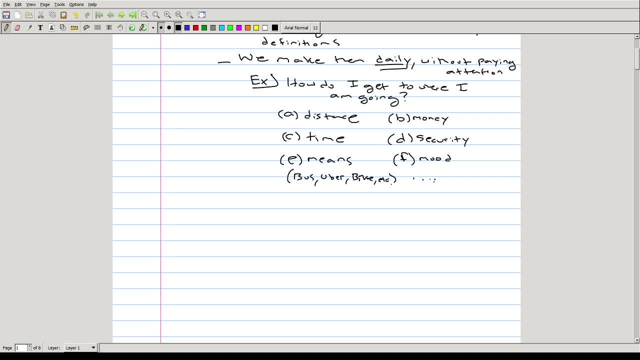 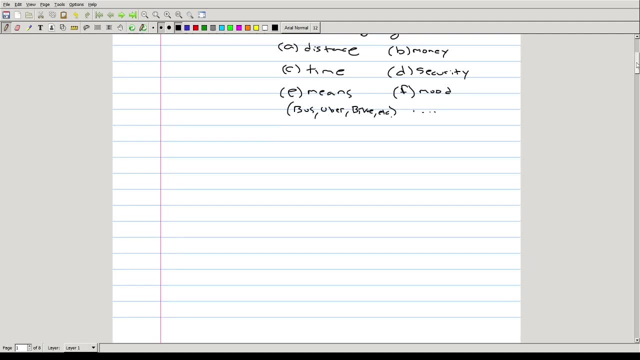 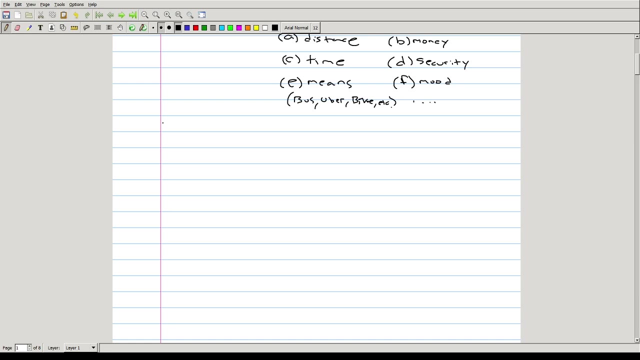 without even realizing it sometimes. So to put a definition down to mathematical modeling is not necessarily the easiest goal, but again, like I said, I'll try to describe it and a lot of the examples and the material. specifically, this definition that I'm about to write down comes from a very, very, very good textbook from one of my advisors, Meier-Humey. 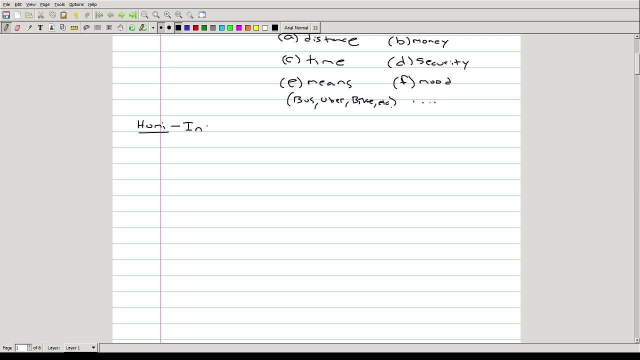 and this is the textbook Introduction to Mathematical Modeling, And if you're going to get any companion textbook for this course, I would recommend this textbook, in addition to the others that I've provided in the syllabus, because this is a fantastic, fantastic overview and in-depth look at many of the modern aspects to mathematical modeling. 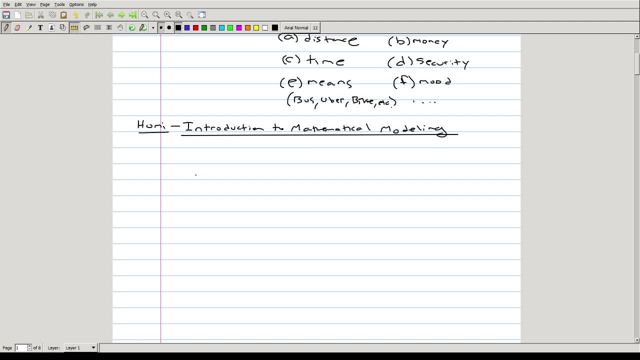 Thank you, But right now I'll write down the definition to mathematical modeling given in his book. In general, modeling is the art of describing in symbolic terms the language. This is where your mathematical and physics theories come in a real-life system. 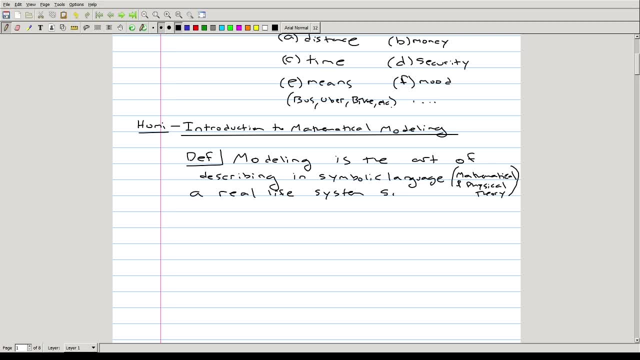 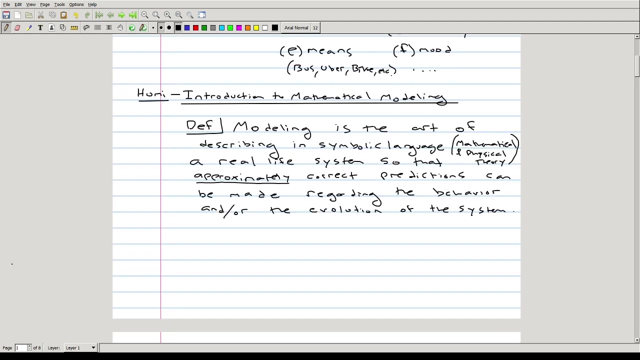 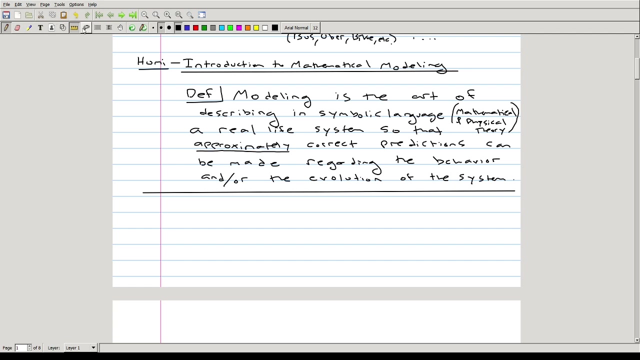 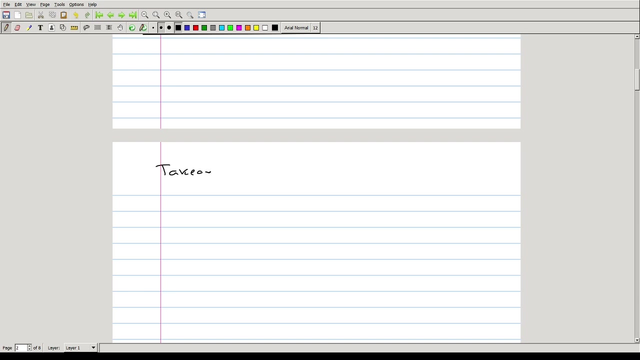 so that approximately correct predictions can be made regarding the behavior or the evolution of the system. and there are a number of different takeaways here that we want to make from this definition, the main ones being that modeling is an art and there are no rigid rules, and what that means is that there are no rigid rules. 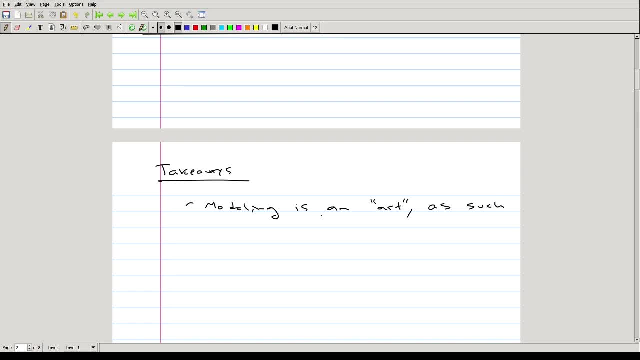 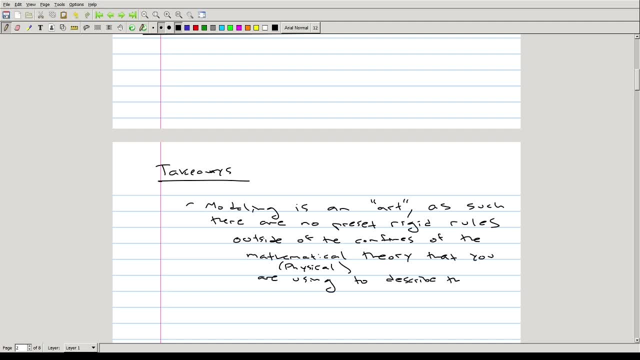 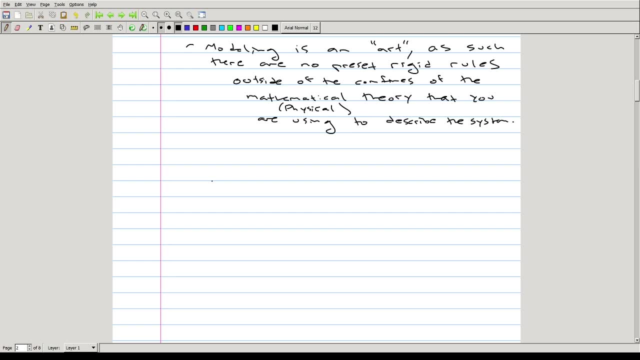 to describe the system, And this is a very, very important point. It really is an art, and it's an art that you kind of develop over time, so you become better and better at it over time and with time and practice, And I also want to point out that, however, here there are patterns. 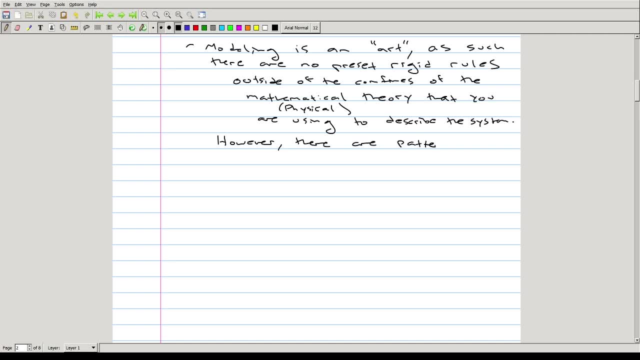 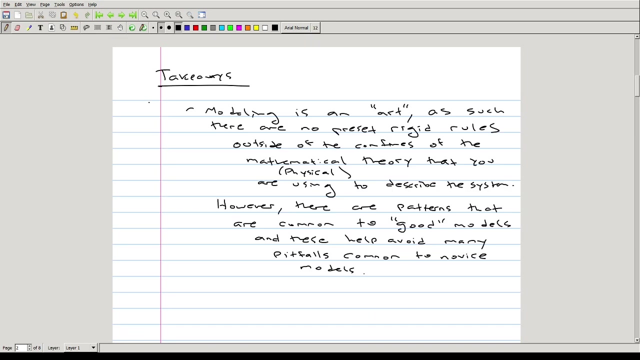 Okay, These are patterns of best practice that are common to good mathematical models, or to just good models, Okay, And these help avoid many pitfalls that are common to creating a mathematical model. Okay, The other takeaway that I want to give you and that I want to point out about this definition: 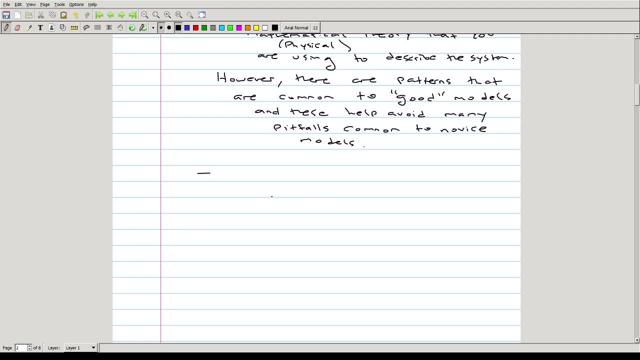 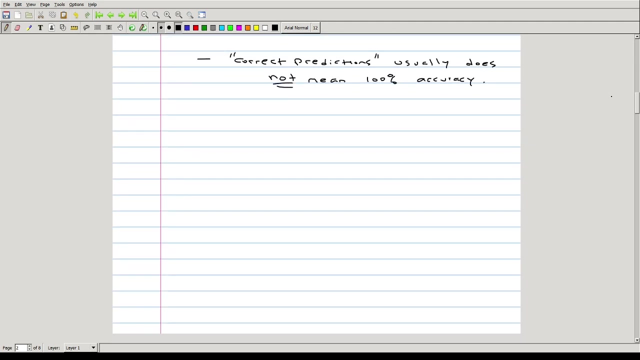 is that correct predictions usually does not mean 100% accuracy. Okay, Yes, Okay, All mathematical models have limitations and, as such, it's up to us, who are the creators of the model or those creating the models- Okay, models- to clearly state and investigate these limitations. 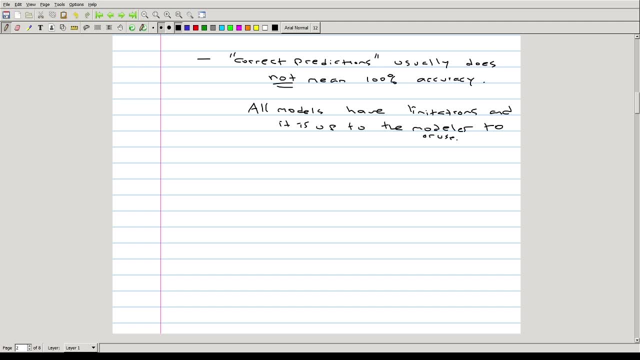 You should also put the user here as well, because many times you can use a mathematical model and not be the creator of the mathematical model. But regardless if you're using a mathematical model or you create one, you have to determine the limitations and clearly state the limitations. 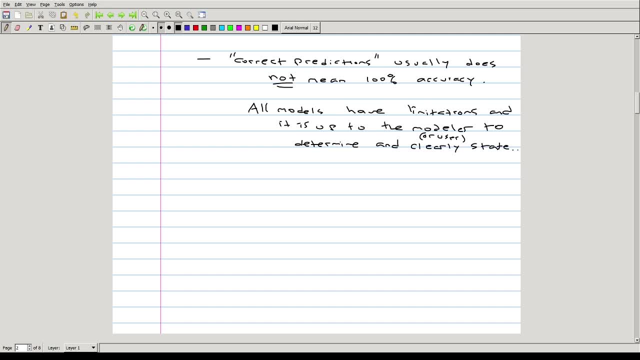 The other thing that I want to point out when it comes to these correct predictions is that sometimes several models describe the same phenomena With varying degrees of accuracy and complexity. Sometimes a model that is too complex may be a more accurate description of reality, but be very, very hard to apply. 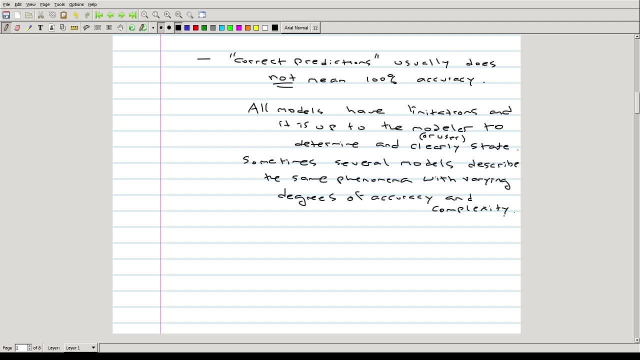 And a simpler model will actually describe the real life phenomena in an accurate enough way and it'll be good enough. And what I want to do is give you a very, very, very good example of this, One example, And this is the example- of gravitation theory, the theory of gravity. 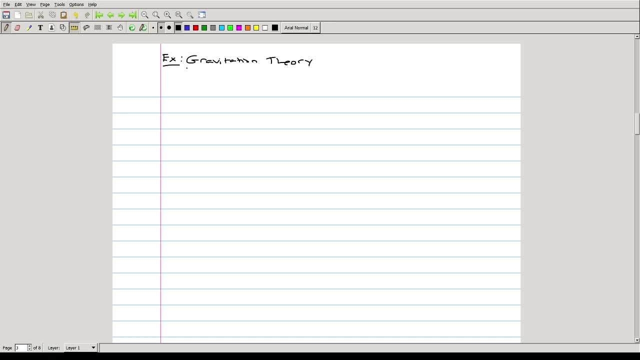 And there are two main theories of gravity. There are many theories of gravity that have been developed, but the two main theories of gravity that have been developed by physical scientists and by humanity are Newtonian theory of gravity, or Newton's theory of gravity, And that of Einstein's theory of general relativity. Albert Einstein. 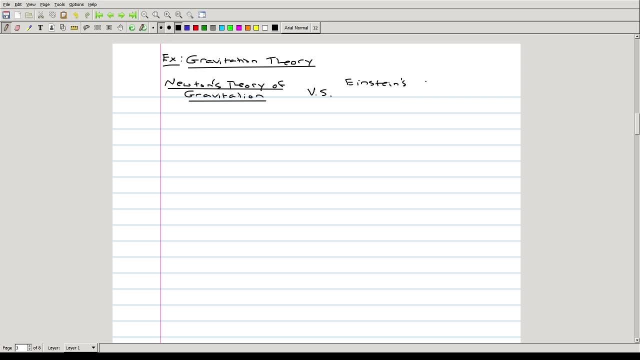 Thank you, And I'll also include- because I glued special relativity over here, I'll include Newton's theory of mechanics and gravitation. So we'll start out by comparing and contrasting these two major developments in scientific understanding Of mechanics and gravitation. Newton developed his theory around 1687. And there is some controversy between whether he discovered parts of the theory and others discovered parts of the theory, like Robert Hooke. But we'll avoid that controversy for now by just saying it's Newton's theory of gravity. 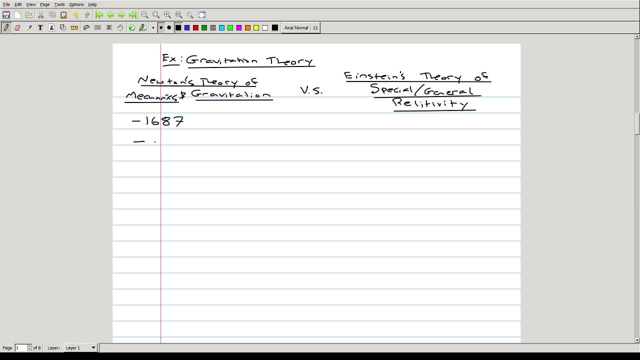 And start out by saying this is an extremely successful theory of mechanics and gravitation. It was so successful, in fact, that this theory was actually used to achieve the moon landing In the Apollo missions, which is one of the biggest achievements of mankind. 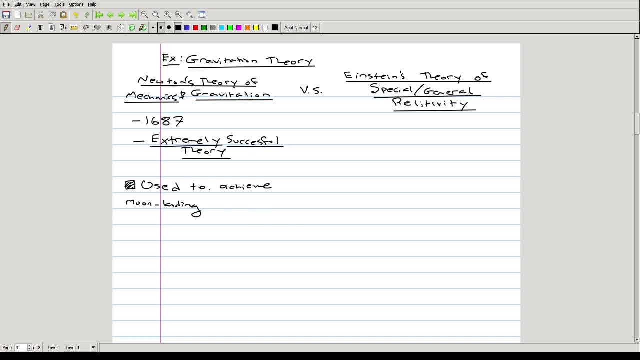 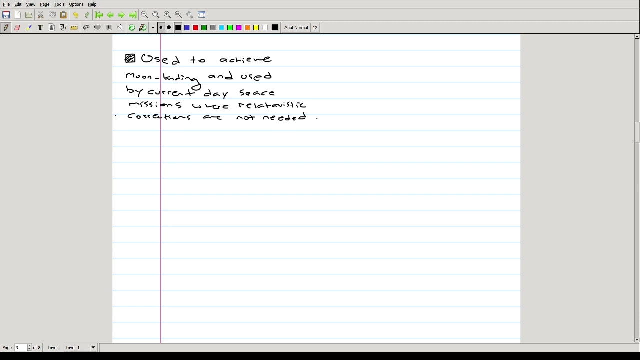 It is also used by current day astronomers and astronauts. in current day missions where relativistic corrections are not needed, We can use Newton's theory of gravitation to actually prove, mathematically prove- Kepler's three laws, And this is something I do in my graduate engineering mathematics class. 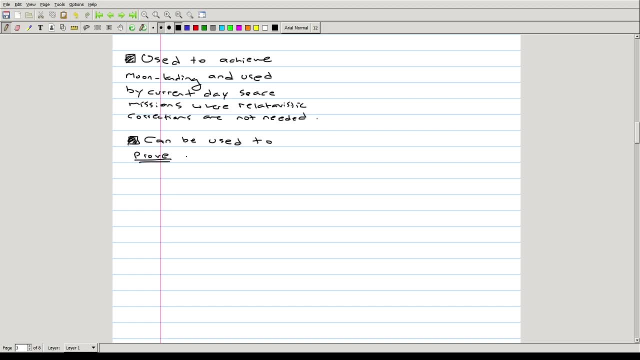 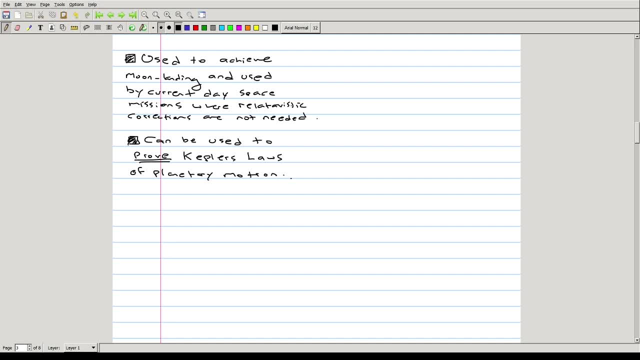 They also relate the area of traversal to the period of motion and give you a relationship between the period and the length of the semi-major axis of an orbit of a planet around a massive body. This theory is also easier to apply and use than relativity. 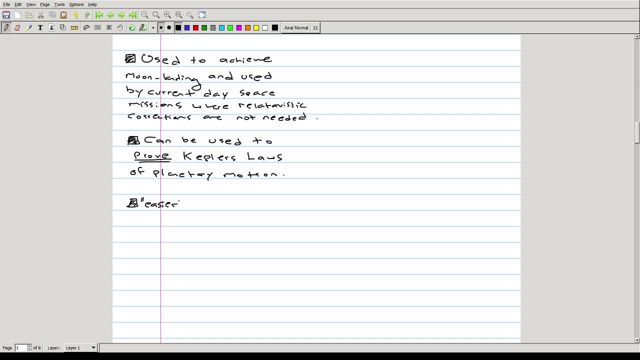 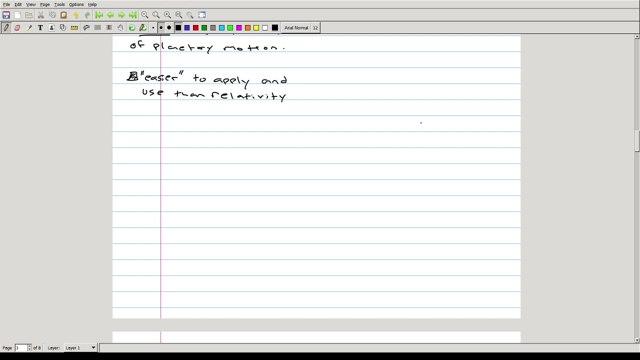 I put this in quotation marks here because there are some caveats, but in general it's much easier to apply Okay And use than Einstein's theory of relativity. However, there are, for all the benefits of this theory, there are some major limitations. 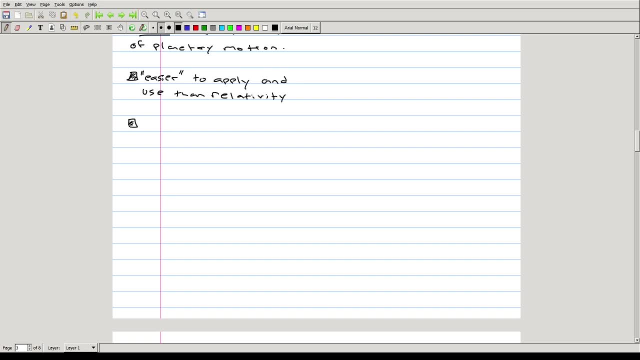 This theory is also easier to apply and use than Einstein's theory of relativity And perhaps you know one of the most historic and biggest limitation was its failure to calculate the precession of various planets, of the perihelion of various planets, specifically. 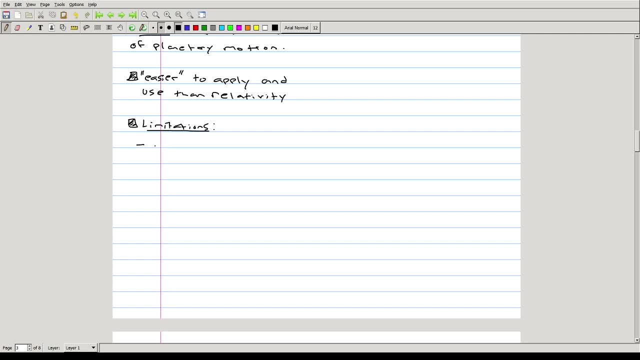 Mercury. Its prediction is way off, But there are a number of ways for us to calculate the precession of various planets. One of them is to draw the diameter of the point V, which is equal to the mass of a mechanism at the end of the space, at the beginning of the universe. 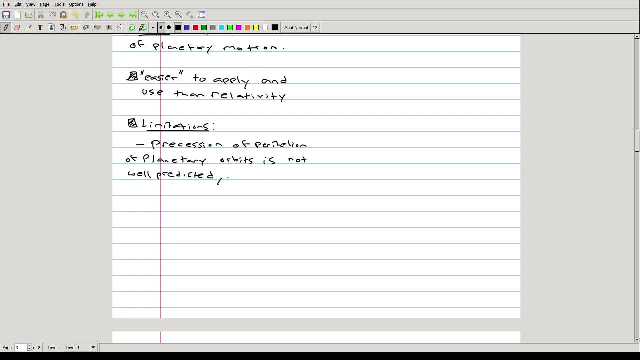 It's not just an ask of an answer, but an answer to a question or an answer of a given question about the magnetic field, the magnetic field itself, etc. The question is: how well do you know the material around us? How do you know if we are on the planet or not? 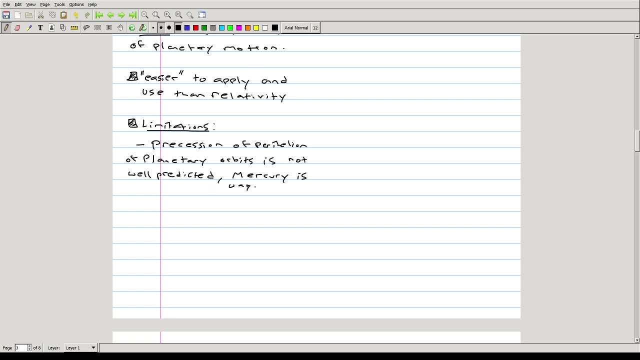 That's a kind of puzzle. Another limitation is that the angular deflection of light or light rays around gravitational bodies is also way off. For instance, if you have the sun here and you're on the earth right here, light rays. 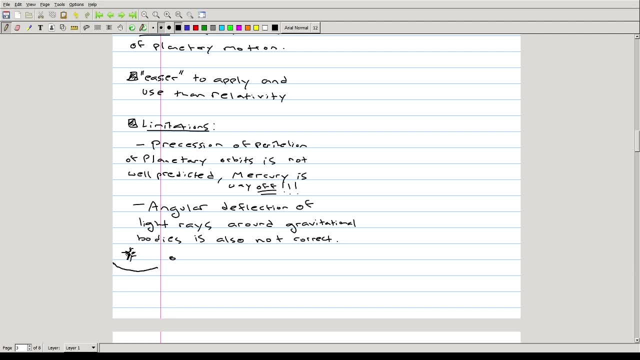 as they pass the sun, if they're coming in like this, end up getting deflected by the gravitation of the body, For instance, if we're looking at the sun, if we're looking at the earth, if we're looking at the sun, if we're looking at the earth, if we're looking at the earth, if we're looking 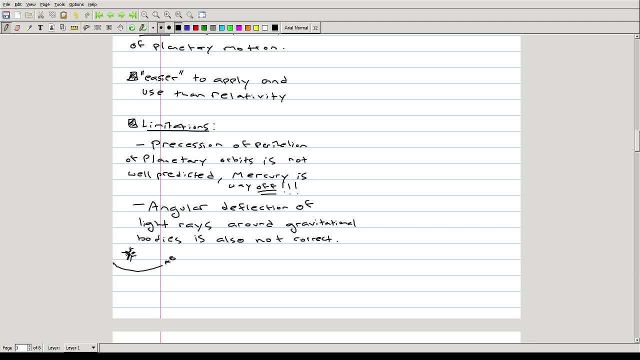 at a star and you see a star in this direction from the earth. the actual location of that star is over here. This is because of the gravitation of the sun. it actually deflects light rays. This is not well predicted at all by Newton's theory of gravity. 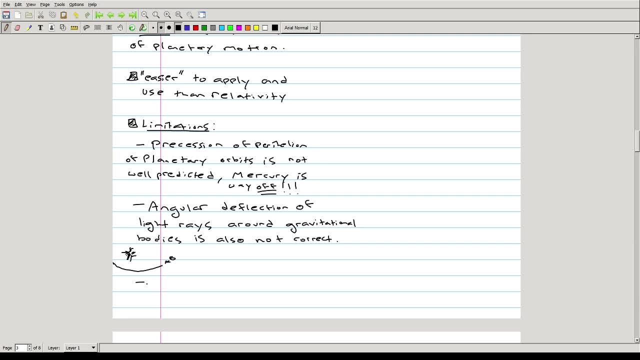 In general for Newton's theory of gravitation, errors build up over time. Here, if we have a half second, I have a gradients vector right here. Here, if I have a half second, and if I have a quarter second, I have a half second and 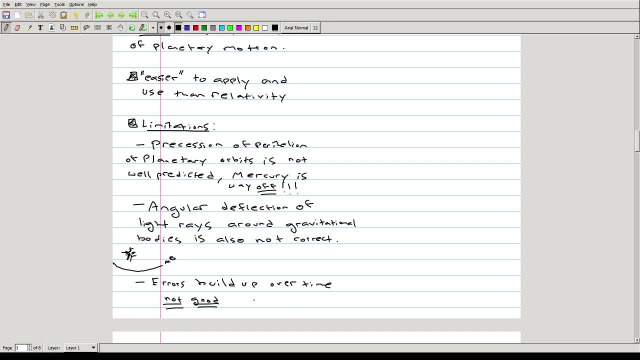 I have a half second, I have a quarter second. this is what I mean. Notice, this is to give you a good idea. I'm now just going to give you a graph of the time when it's all over here, In any case, for long, long course time. this is the first time you're going to see. 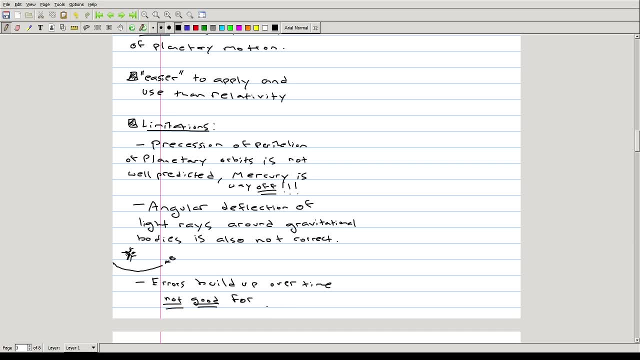 a half second, So they all meet on a half second. It allzear, and so you can see all this difference in time. Look and see if you do get the idea. So I'm going to add a two- Quest which is a distance from the sun, and this is the. 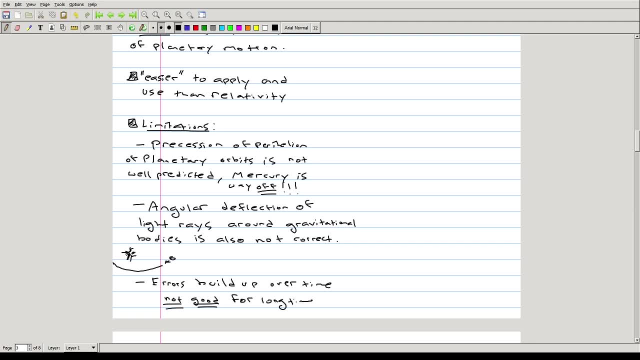 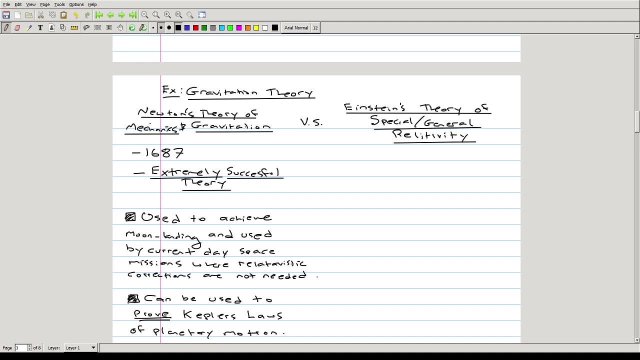 time span, And you can calculate the distance when you do get the data. This is a summary of Newton's theory of mechanics and gravitation. On the other hand, we have Einstein's theory of special and general relativity. Einstein published his papers around 1916, and this is also an extremely successful theory. 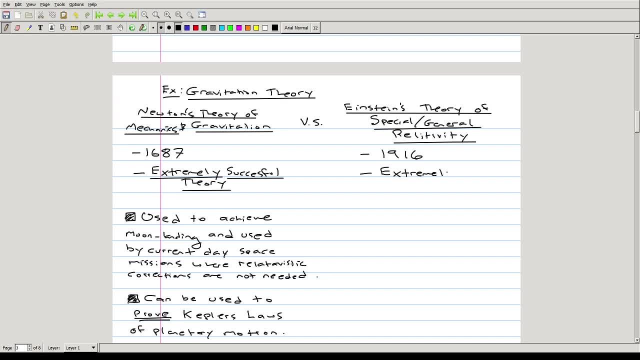 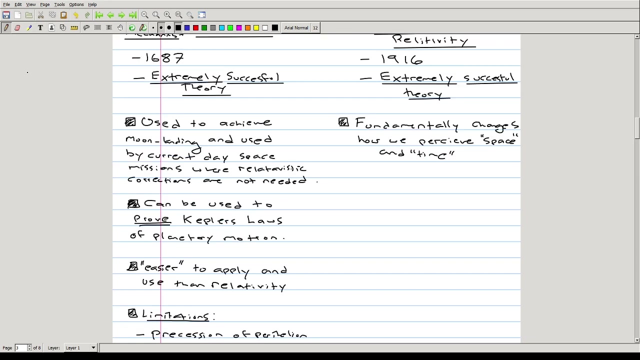 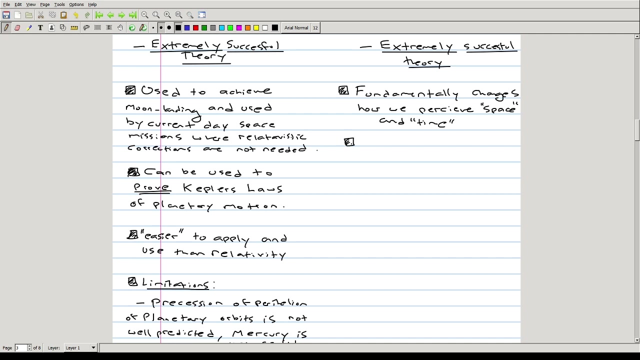 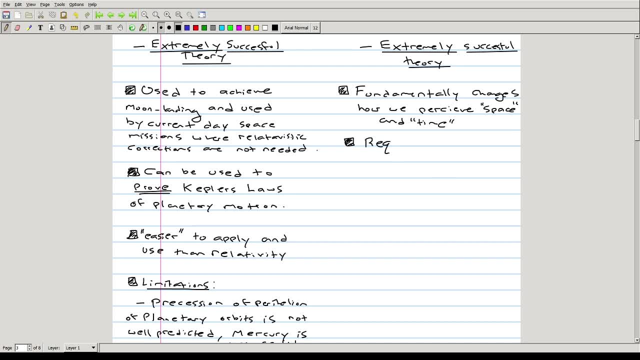 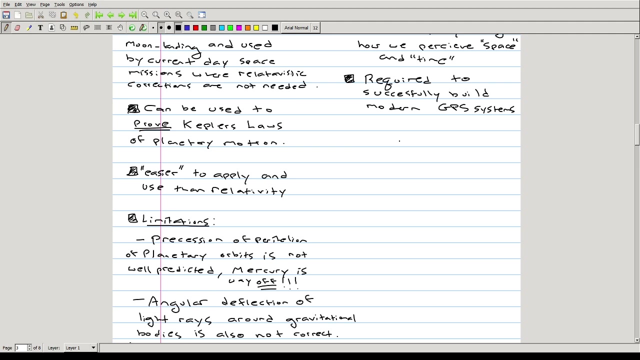 modern systems And in general, by greatly overhauling, recalling a lot of the fundamental ideas of space and time and fundamental ideas in physics. the theory addresses and explains and corrects the limitations of Newton's theory, While simultaneously better explaining why gravity works. 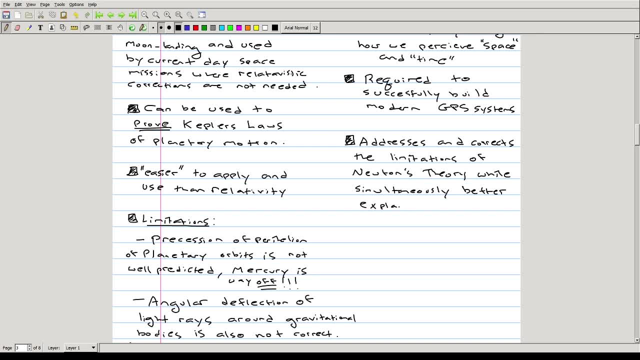 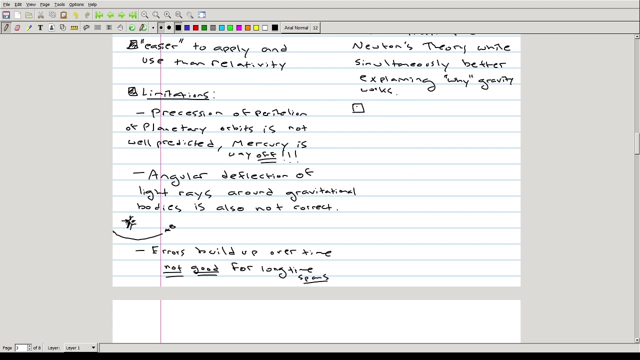 And, in general, it's much harder To correctly understand, apply and solve problems in general relativity. There are definitely some other limitations to this theory as well: Extreme scenarios Such as very, very large mass, Like black holes. 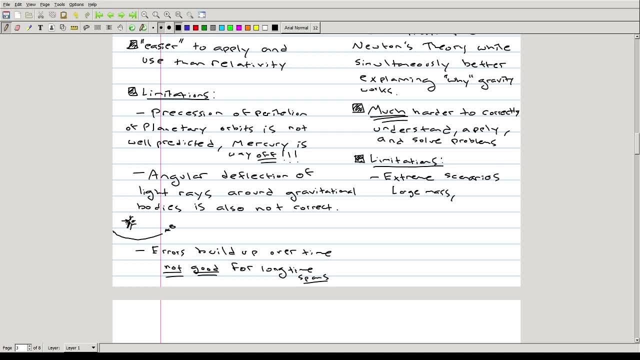 We have complications because there's a fundamental misunderstanding of how general relativity, which works at large scales for very large distances and large scales between planets, interacts well With quantum mechanics, which is the theory of the very small, So extremely small, fundamental particles. 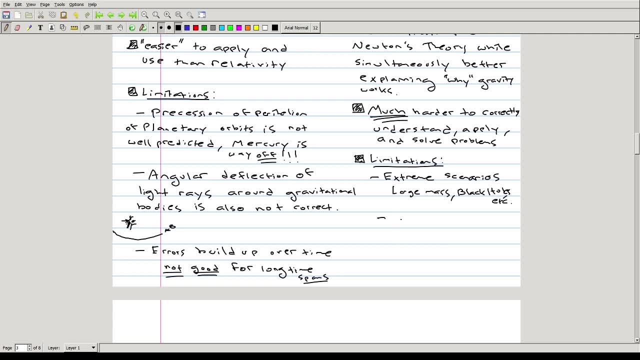 So, in general, Einstein's theory of relativity doesn't mesh well with quantum mechanics, And this is actually one of the biggest problems in physics right now is to find a new physical theory that gives us Einstein's theory of general relativity but meshes that with quantum mechanics. 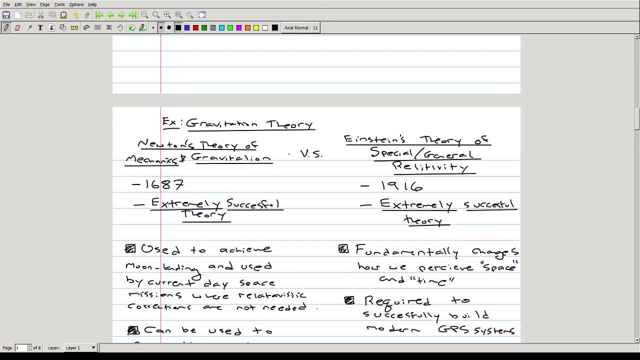 But in terms of just theories of gravitation, the more modern theory- and some people will say the better theory- is Einstein's theory of the special and general relativity. But I wouldn't say that it's better, I just think that it's more modern. 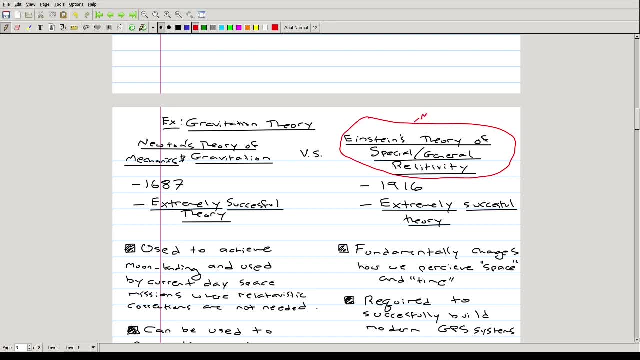 It's more modern and it's more accurate. It's a more accurate theory And significant accomplishments in mankind have been achieved by both theories. World-changing accomplishments have been attained using both these theories. What's also important to note- and this is the final note that I'll make on this example: 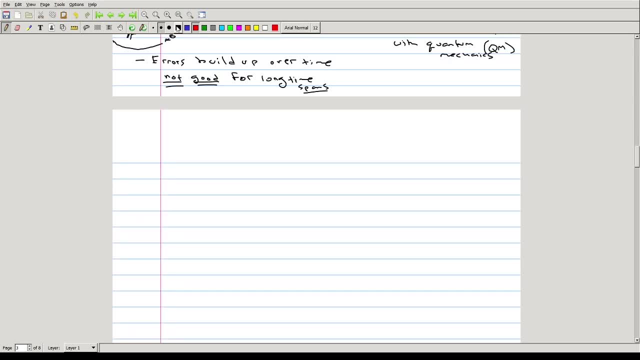 is that sometimes, if you have one theory that's less accurate, one theory that's more accurate, you can address and use the less accurate theory while introducing corrections from the more accurate theory. So, for this example, Newton's law, Or I should say Newton's theory of gravitation can often be used with and is often used with. 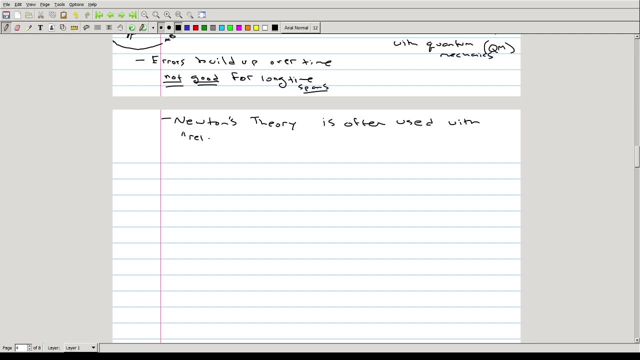 what are called relativistic corrections- Thank you for watching- attacked on- or attach, which will correct Newton's laws and add in the corrections that we know are actually true and observed in real life. that can be explained via relativity And we'll investigate this a little bit later on. 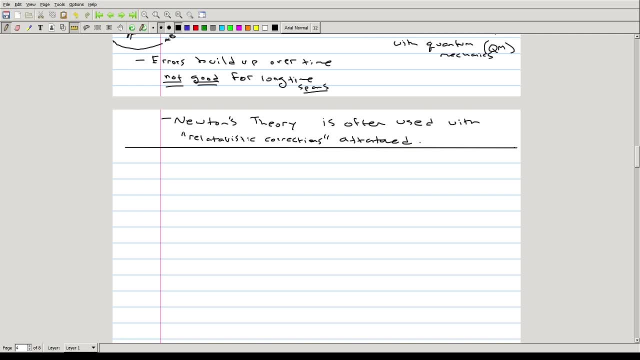 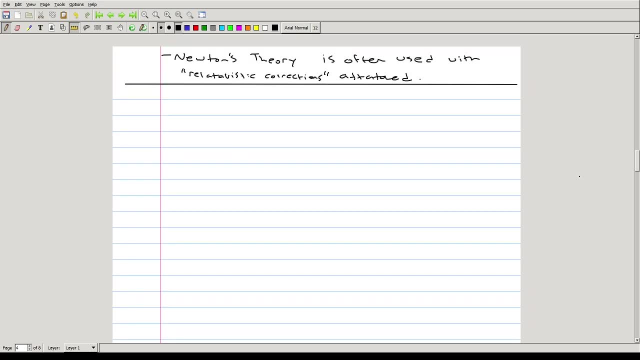 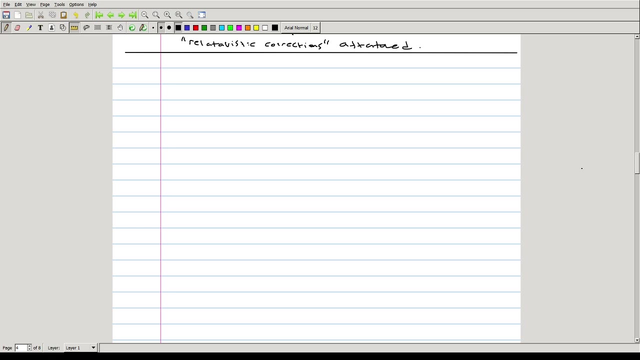 in the course, when we get some development into our toolbox, our technique. But the main thing you want to be thinking of in this course and in general when you're learning mathematics, is how it's adding to your toolbox for mathematical modeling and for figuring out problems using mathematics. 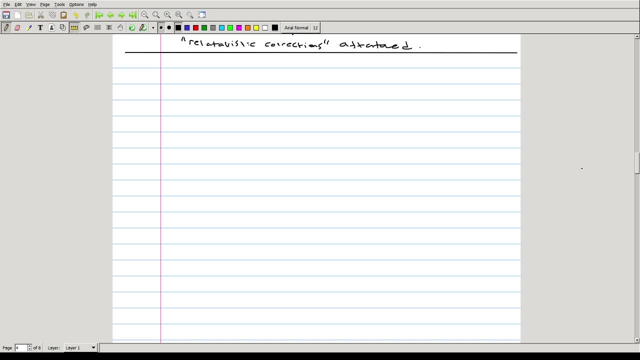 So what I want to do now is just give a a quick overview of the general modeling framework and what mathematical modeling problem consists of and how it's typically a very large process, So I'll give you my last few minutes here, Thank you. 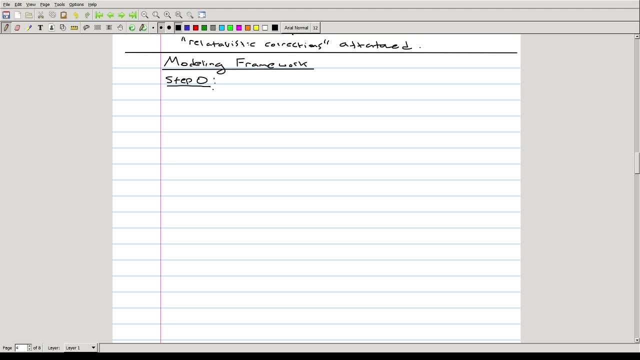 And, just like the previous definition, this process can be found in Meyer Hume's book and I very strongly recommend taking a look at the book because it's a very, very nice and very, very nice book. It's a very, very nice book. 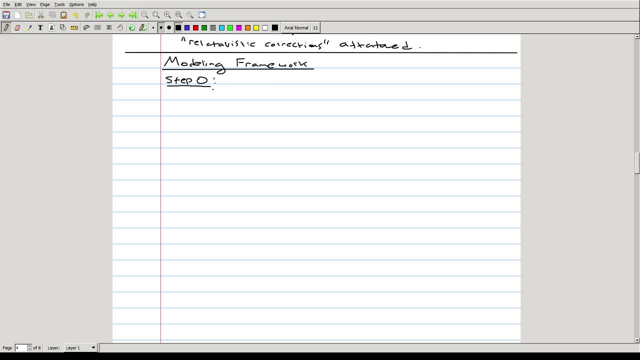 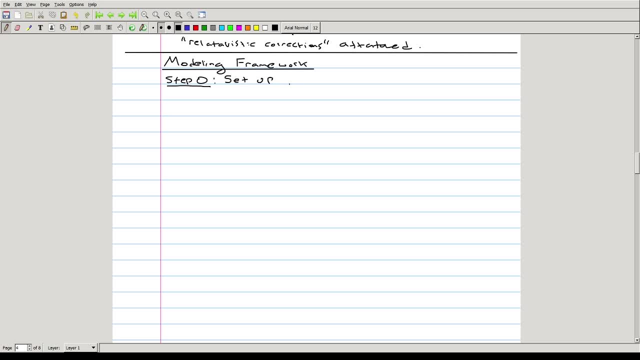 process is to set up as precisely as possible the reasons for constructing the model, the reasons for constructing the model and its objectives. so, for example, if you're making a model of the weather and you want to predict the weather, do you want to predict the weather for a day you want to predict? 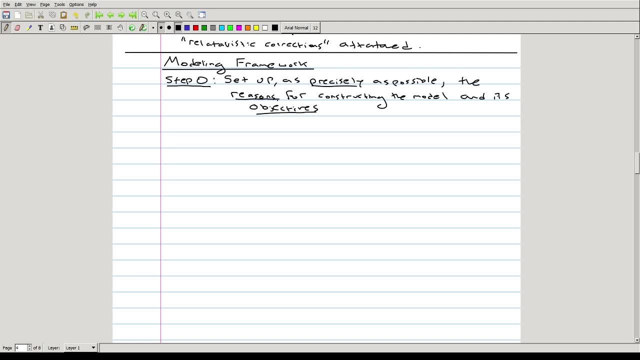 the weather for an hour. do you want to predict the weather for a week? right, each one of those questions is a different question. it's a dip. they all are very difficult questions, but they have very, very different difficulties associated with them and, as you can see, if you look at your local weather forecasts, you don't really get. 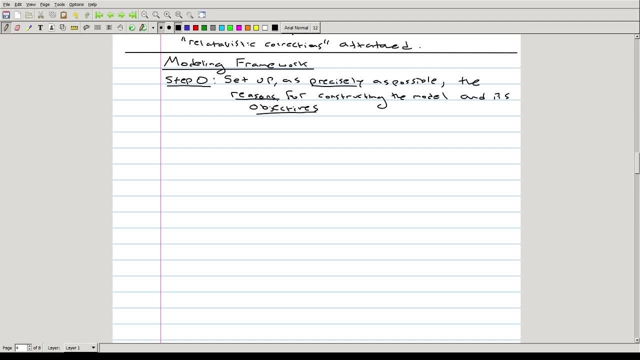 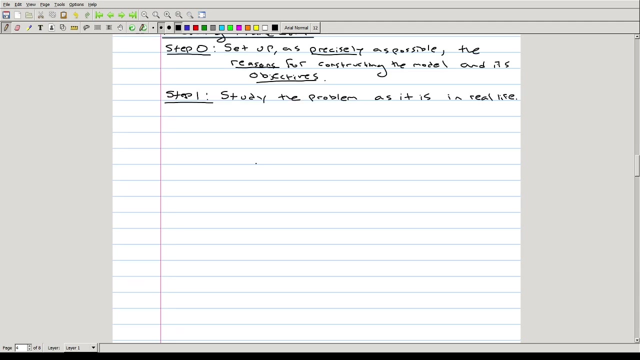 much accuracy, even within a few days, for weather forecasts. so one set one is to study the problem as it is in real life, and this involves doing that essential work. this includes skills, lot of research to figure out exactly what the problem is you're dealing with. 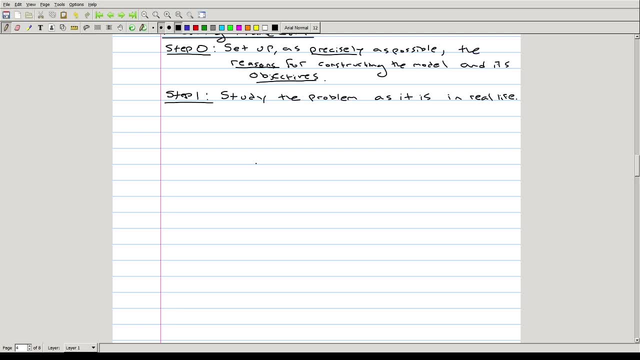 and you know what exactly is going on. it's also setting up for the next step, step two, which is data collection and analysis in real life, and this is where you go out into the field, or you, you collect data from laboratories and you, you, you, you collect real world data to analyze. 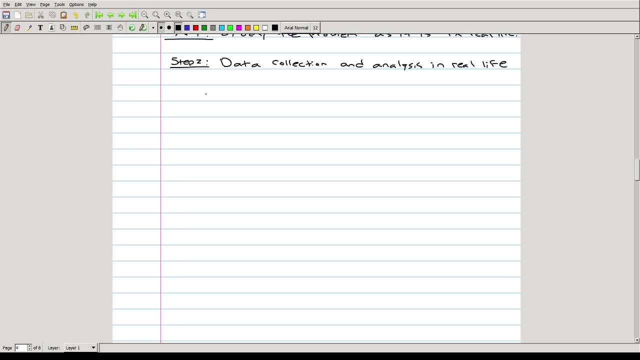 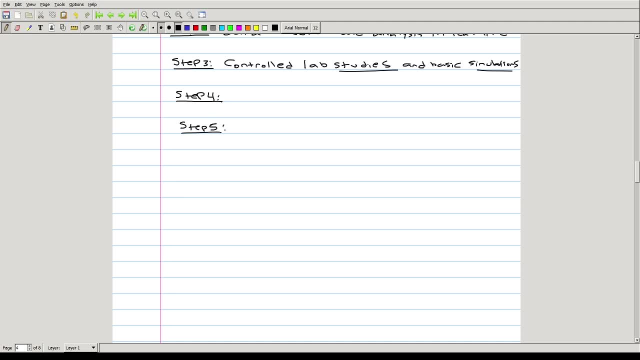 step four and step five: step four- barrier blocks into market. step four: step four- barrier blocks into market is the construction seats to to select a different, unique type of一個 of a conceptual qualitative model, And notice that I'm using the word qualitative here, not quantitative. 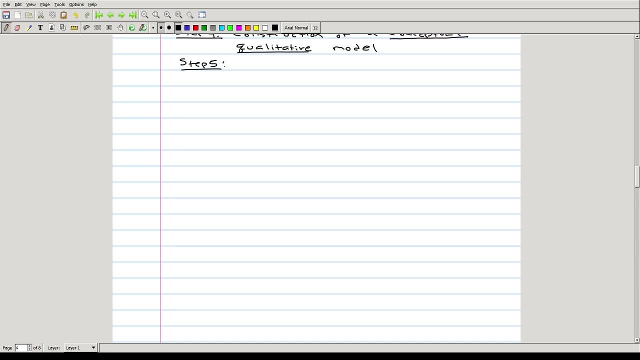 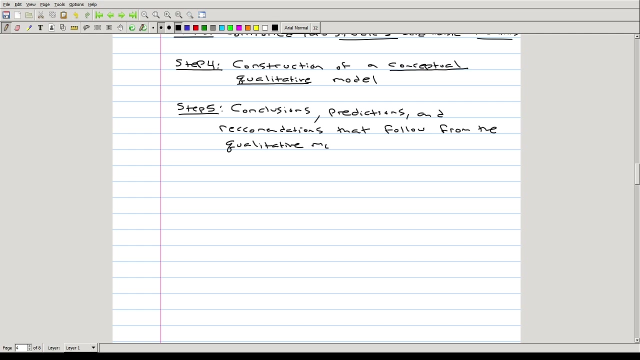 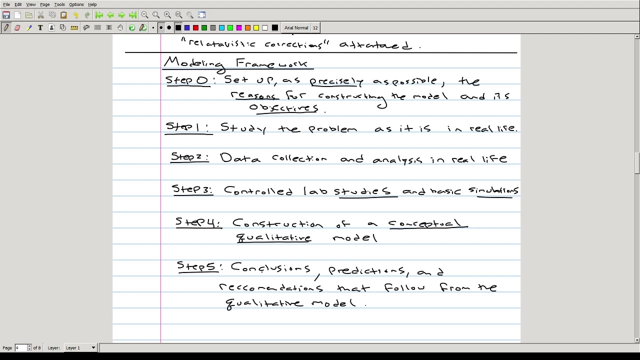 And the last step here is conclusions making, conclusions, predictions and recommendations that follow from this qualitative model. And that's the last step of this process, Thank you. And these five steps form the basis of a given model in science, But essentially, these steps are very often not enough. 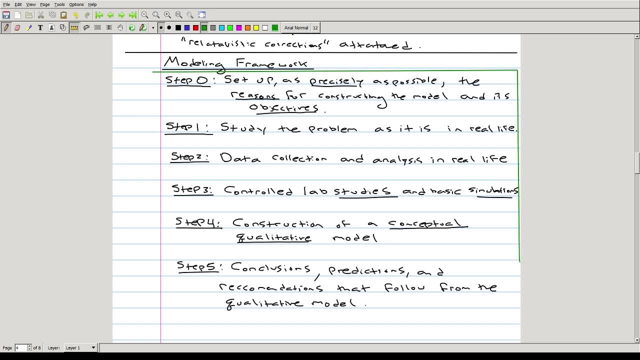 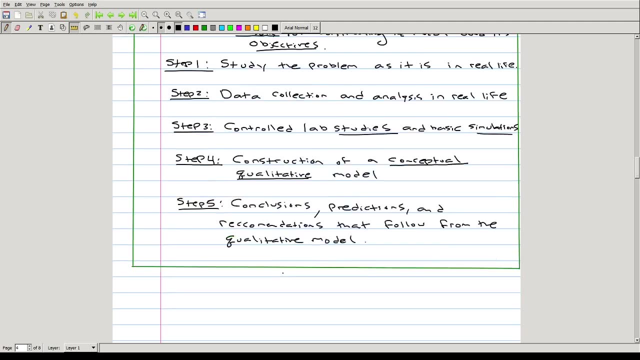 Right, This is a very important step. This is a very important step. These steps are only the beginning of the modeling process. So these five steps- I've just made a box around these steps- because they all together form the basis for what's called a qualitative model. 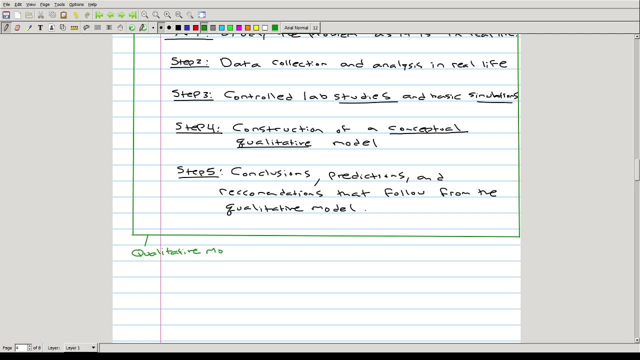 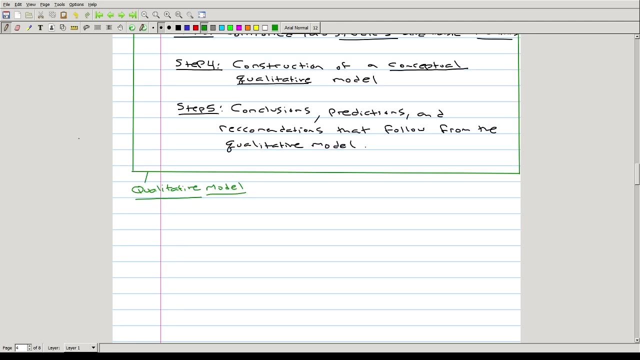 And these are used very, very often And they are useful and can be useful. But it's important to point out that, while qualitative models are, you know, they are extensively used in the social sciences And these are more available today. So you can slightly change the we would say uhkeepers, like potentials, is an easier way. 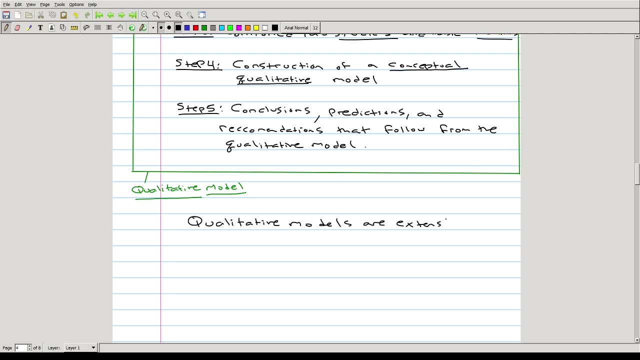 But, uh, yeah, these are similar And this is real here- a very much another, uh, concept of gravitation, of how quantitative models are used for, Okay, Everything. So, um, and actually I want you to really object to the idea that, like the cheatingottoes, 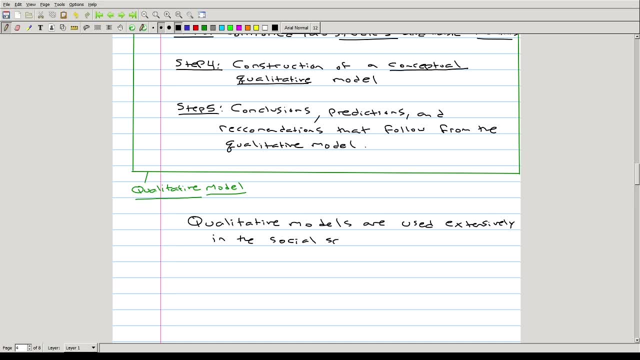 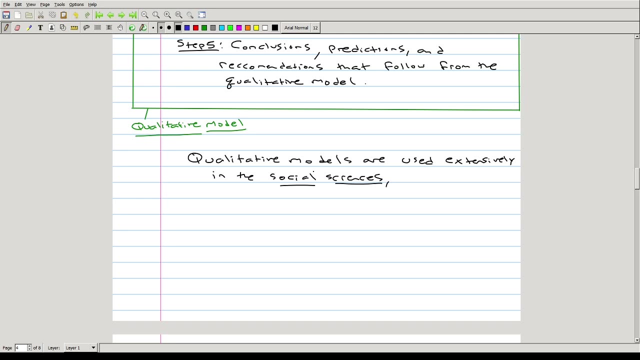 which you probably don't think about it, but are positive treasures, And they're also used in the physical sciences, the natural sciences and engineering as well. But it's important to find, it's important to point out, that they are rarely accepted as fact in the natural sciences. 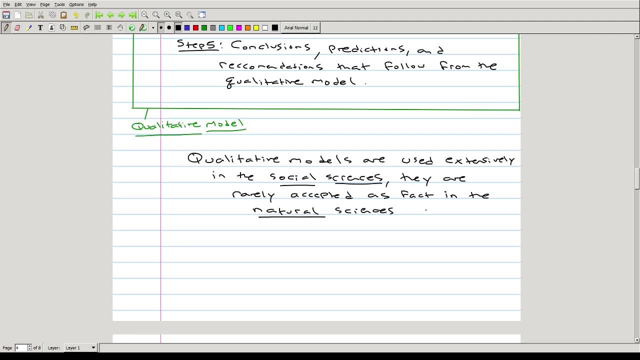 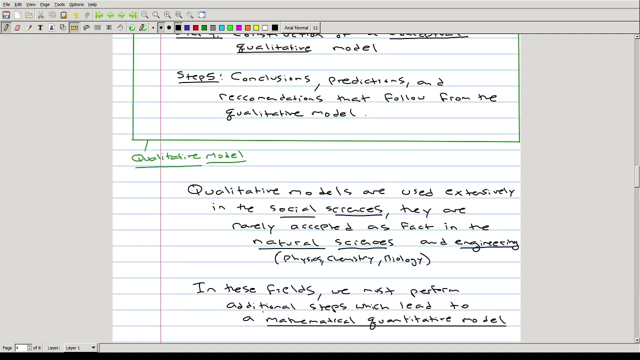 And by natural sciences. here we're talking about physics, chemistry, biology, etc. etc. In these fields we have to perform additional steps Which lead to a mathematical quantitative model- And notice my use of the word quantitative here Rather than qualitative. 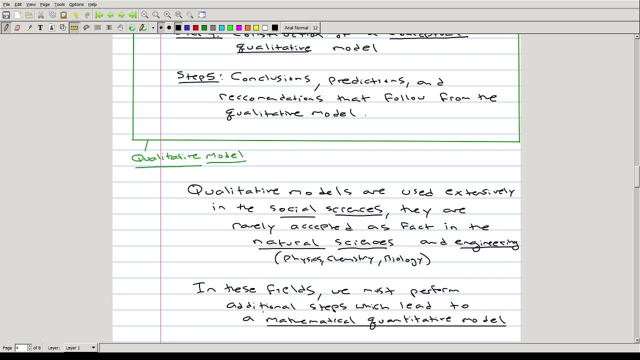 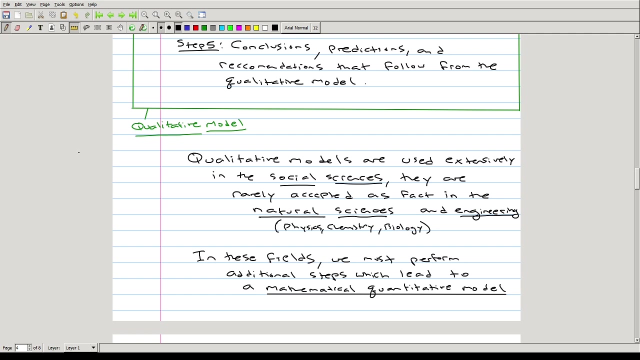 So forming a qualitative model is very often a very useful first step and very important when constructing a given theory, A given physical theory or a given mathematical model. But we need to do more, as natural scientists, engineers and applied mathematicians, to construct real world models. 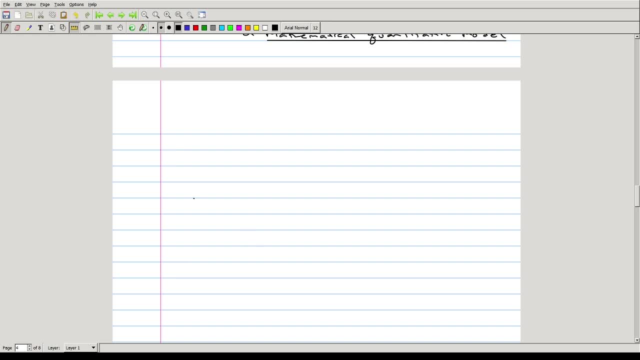 And this is where step six comes in. And step six is the step where we do abstraction and symbolic representation. Look for RGB. And if you don't have an interpreter, And if you have an interpreter, So what'd we do? Let's do one second. 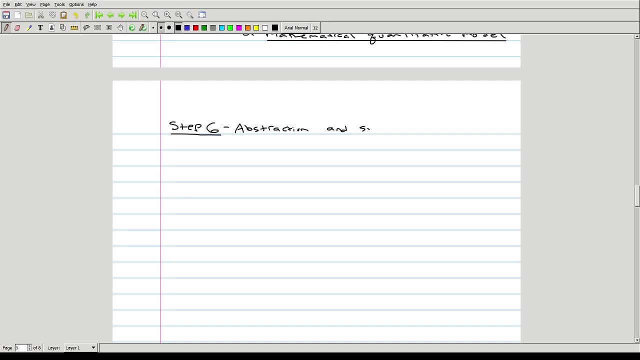 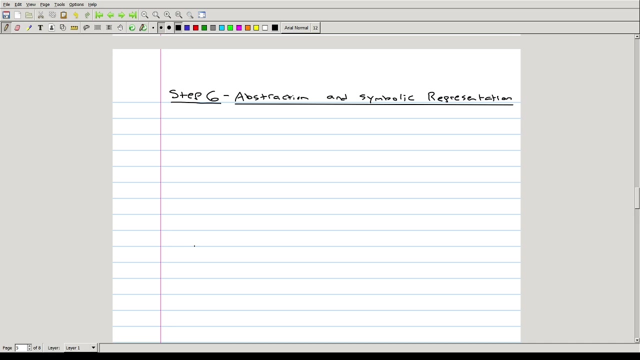 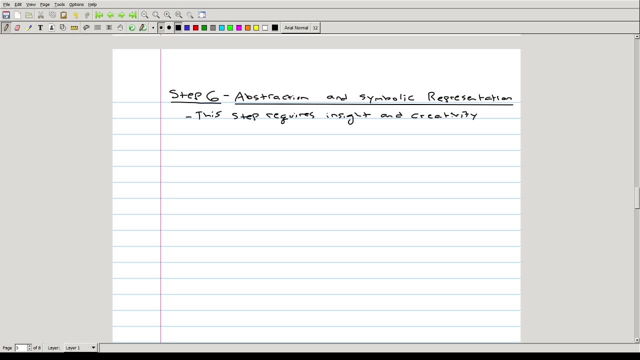 And the reason for this is that typically, the true variables which control phenomena are often masked by the data. So let's take a look at step seven And do many of the amazing modern data science algorithms that have come about, But typically requiring or trying to find out what the true variables are which control a certain phenomena. 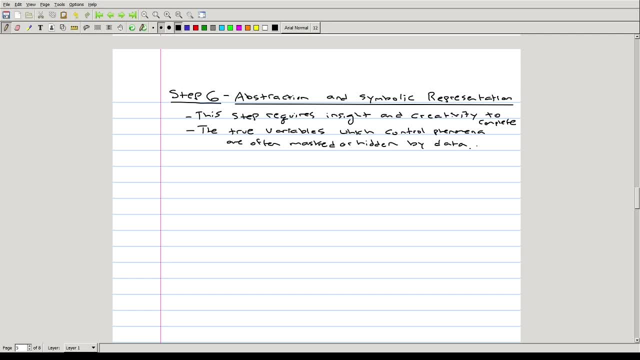 involves a large amount of insight and creativity to come up with a correct symbolic representation and model, And this is also where this step is, where a good knowledge of modern mathematics and the physical sciences is often crucial. And these are my comments on this step. 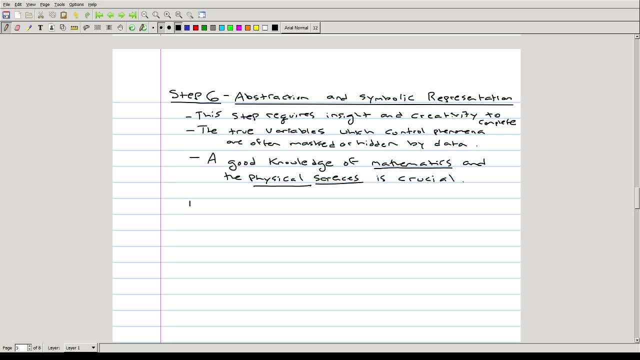 But essentially it consists of representing variables by symbols, naming the functions or other mathematical relations that relate the symbols and that are going to be used in the model. 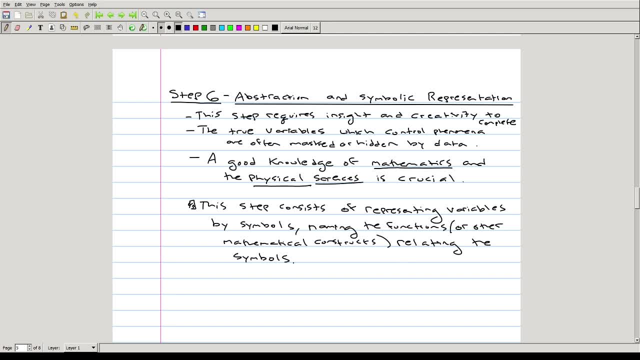 In identifying the axioms and or constraints of the model. 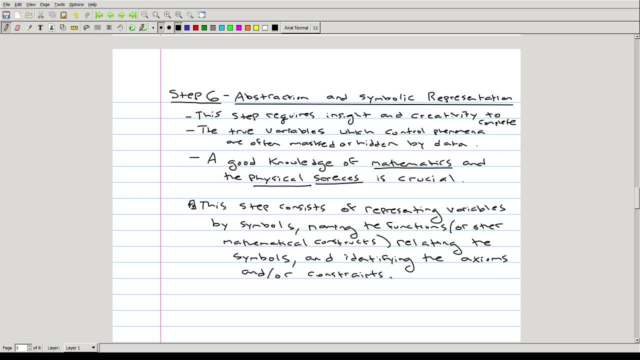 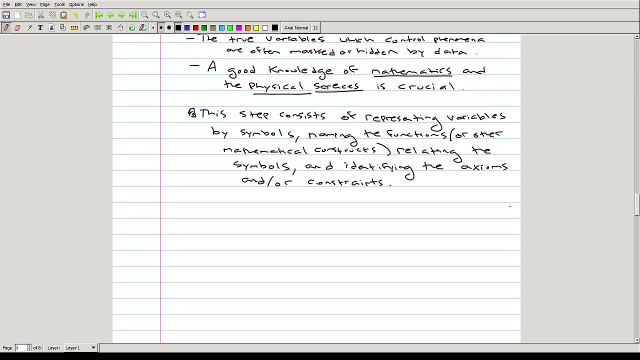 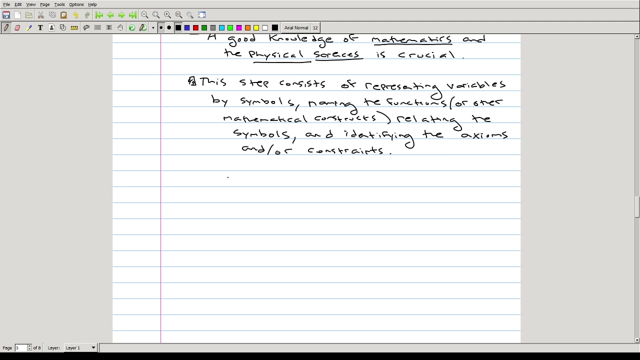 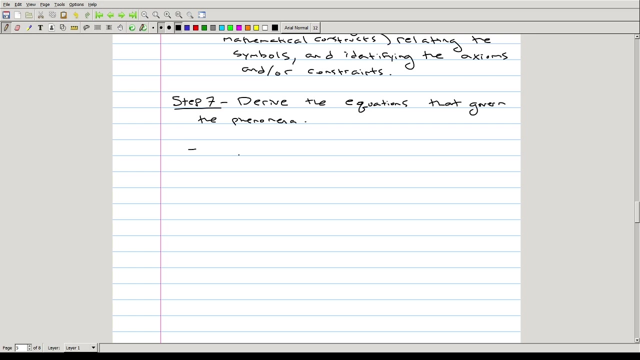 And this step immediately jumps into the next step, step seven, which is to derive the equations that govern the phenomena being studied And some good questions to ask. here are the general classifications of types of models. Is this model a stochastic model? 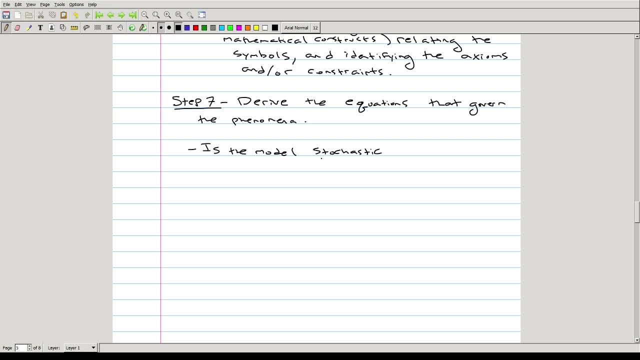 Or probabilistic, Like, for instance, quantum mechanics. is Or is the model deterministic? Okay, Okay, This would be general relativity. So stochastic means there's some degree of randomness in the model and you have to use probability theory very heavily in the model or deterministic meaning. you can always. 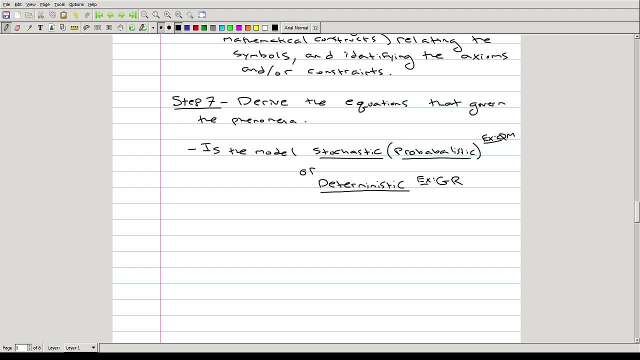 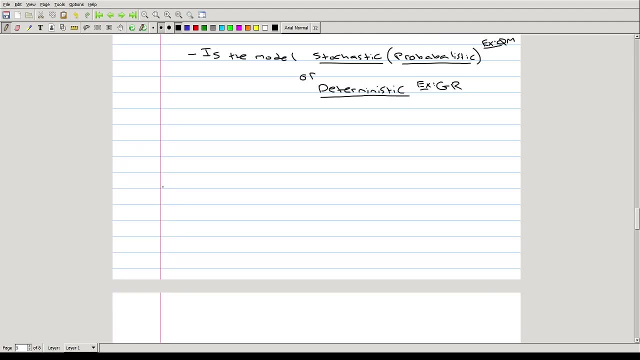 find, in you know, exact trajectory or an exact solution? uh, or is it a mixture of both? this can happen sometimes. another big question to ask is: is the model continuous? so you'll be? will you be using techniques from calculus or topology to discuss the model and solve problems, or discrete? 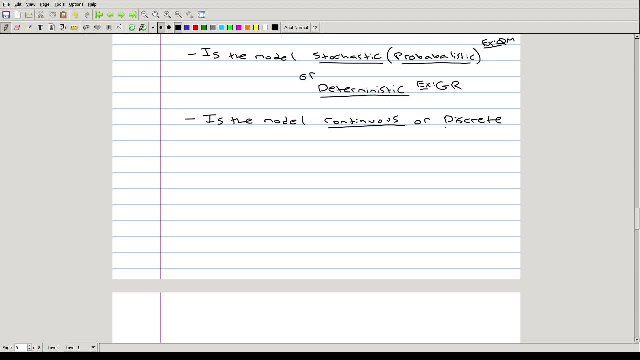 meaning you'll be using methods from discrete mathematics, or like basic helemaalabundance uh mathematically, or pieces from the other side uh logic. In every case, you'll be using logic. The idea is, you know, both continuous and discrete models have large applications and a large 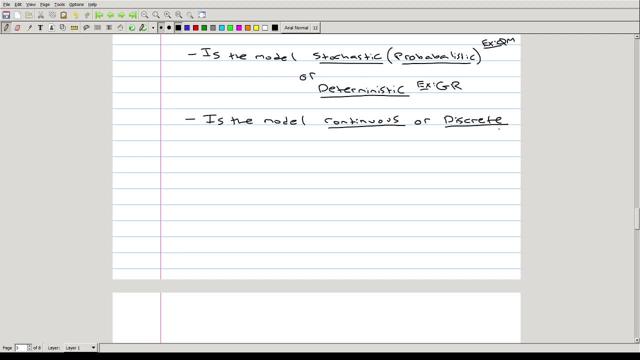 spectrum of applicability to real-world problems And, just like before, you can say: or is it a combination of both? There are many models that require you to consider both discrete forms of the model along with continuous forms and combining them. The main idea here is that 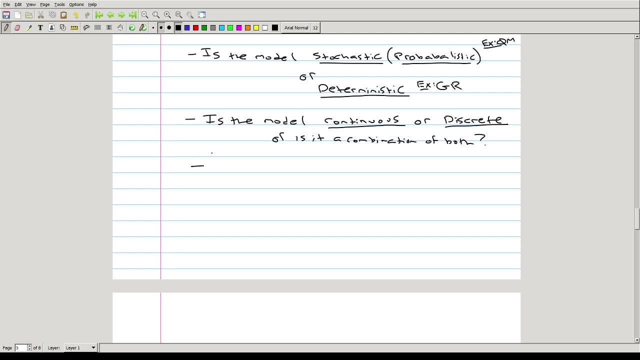 the main idea here is that this step is where the mathematical methods used must be precise and correct, So you have to correctly apply mathematics in the mathematical theorems that you're going to use, in the confines of you know the mathematical construct that you're using. 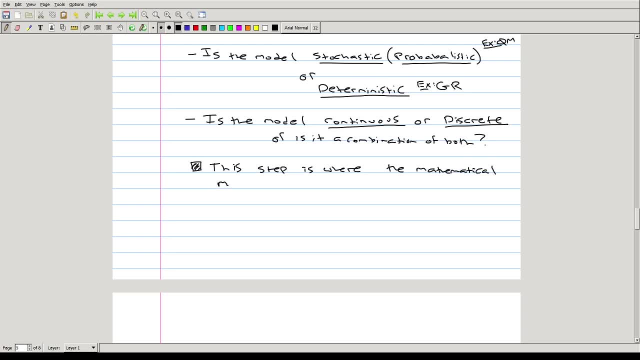 Good, No, no, no, no, no, Excuse, No matter what. okay, So five a times two and 1.. 5, 5 times 2 plus h 1, 1, 1, 0.. 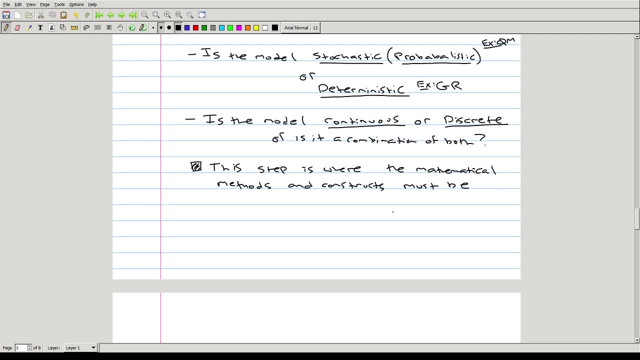 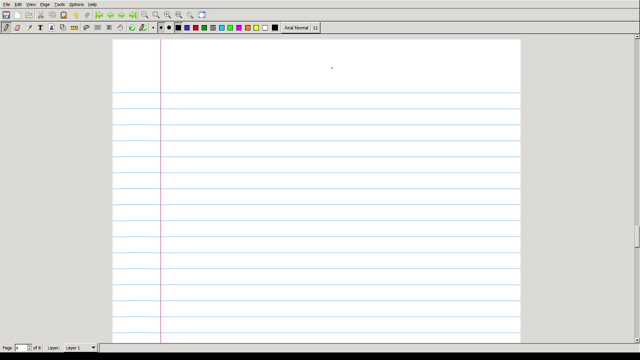 So, to sum up, this ellas, and that these are thearial measurements that I have, noodles are easily overal unique because you have the notes in the formula, there won't be as much interview Till then. thank you all. Once you have your mathematical model and you've completed steps 6 and 7, you'll move. 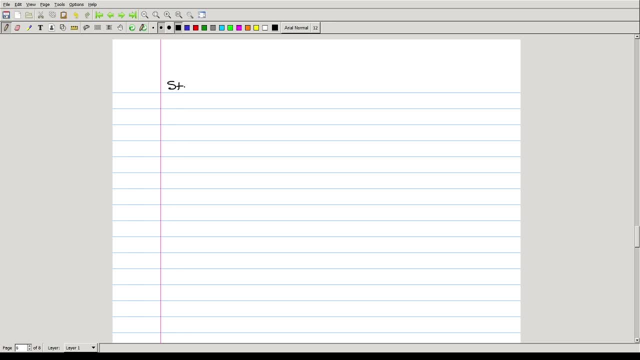 on to step 8, which is model testing. This is the meat of this process. Probably the most difficult and also the most rewarding part of this process is finding solutions to the model from step 7.. And not just finding solutions, but comparing solutions to the model equations. 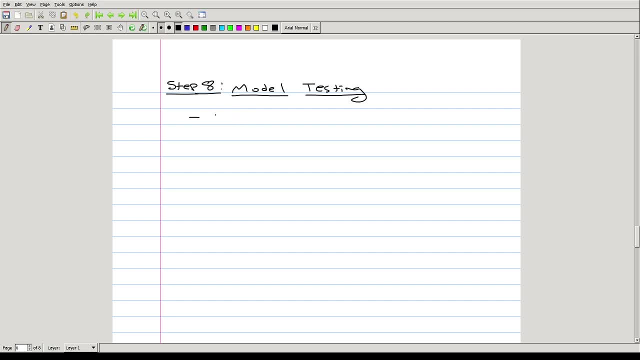 We compare. Okay, Thank you. I'd like you to take a moment to reflect. Okay, Did you have a great session? Yes, Okay, Thank you everyone. Okay, Thank you, Thank you. Bye-bye, Bye-bye. 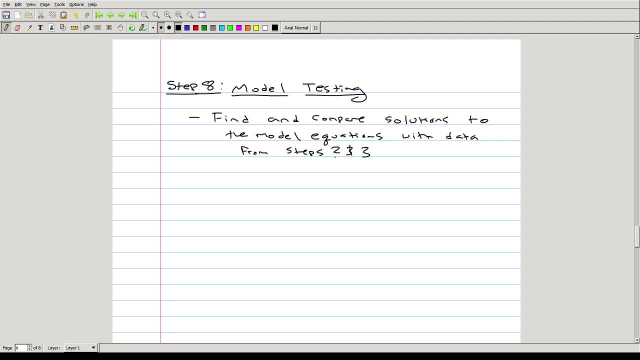 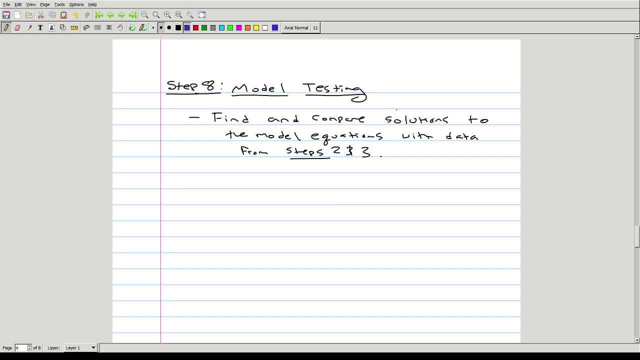 and, generally speaking, solutions here mean a number of different things. but in this class- and as you you might have seen if you talked about numerical methods at all in your normal ordinary differential equations class or in your linear algebra class, solutions come in two forms typically. the first form is the exact analytical solution. 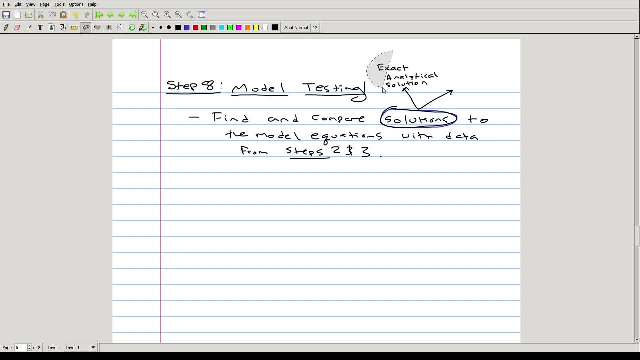 and the second form is a numerical solution or a computational solution. and uh, the, the, the. the numerical or computational solution is uh, typically we think of it as an approximation to the exact analytical solution and um, this in and of itself is a problem. in mathematical modeling is um studying a given numerical procedure, algorithm and showing that procedure, you know. 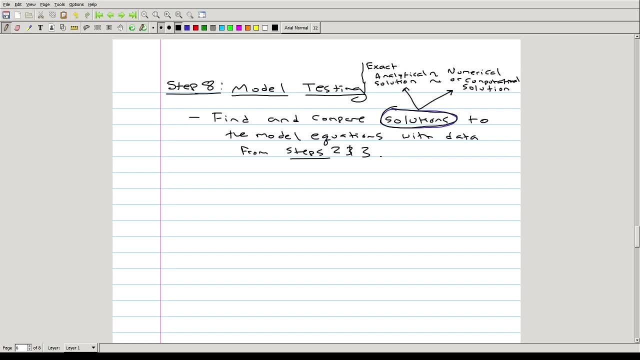 proving that procedure is actually is, uh, correctly approximating the exact solution. this is a huge problem in mathematics. um, i recommend taking a numerical methods course to learn more about this. we will be going over some basic numerical methods in the course and showing how to- how to you do basic numerical methods. 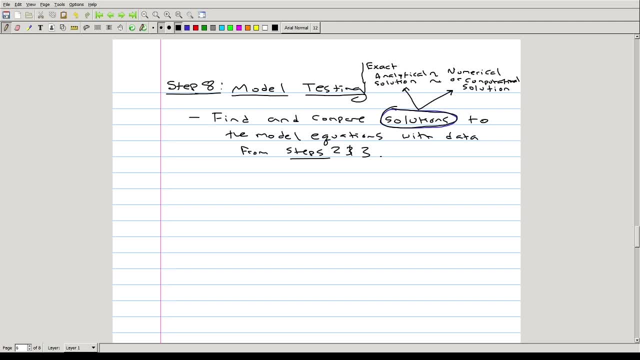 for differential equations. however, i won't be going over them in detail in the course. we'll be focusing more on, you know, getting exact analytical solutions and investigating exact anal analytical solutions. even if we we can't get the exact solution itself. there are many exact methods that have been developed for that, so we'll be talking about that a lot in this course. 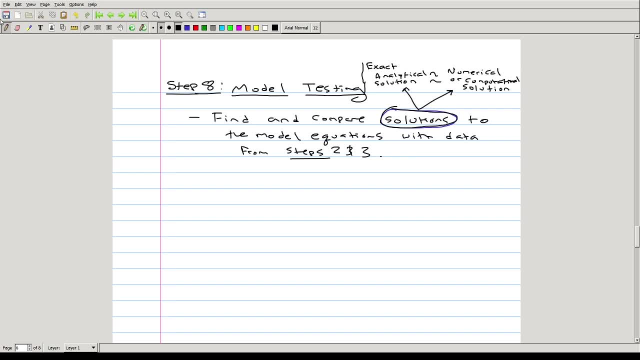 so we'll be talking about that a lot in this course. and it's at this step where- if i in this, you know testing- you have a bad fit, let's say you have a bad fit. and it's at this step where- if i in this, you know, testing- you have a bad fit, let's say you have a bad fit. 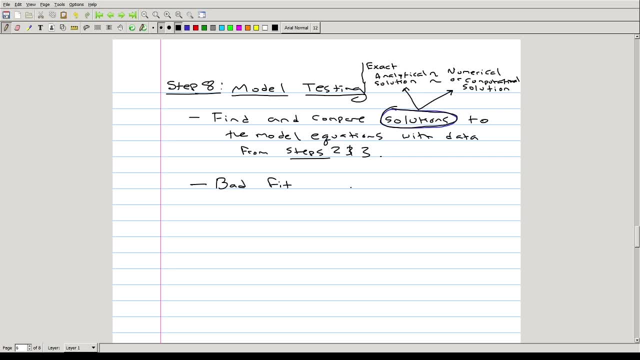 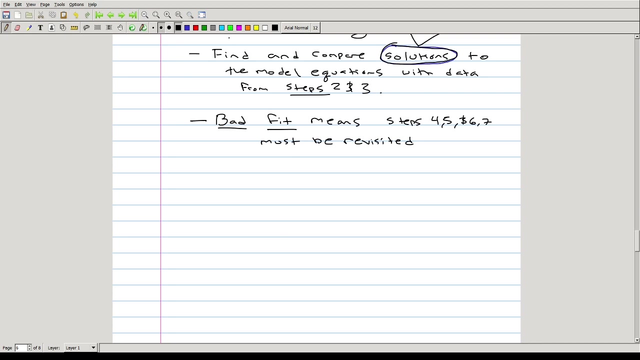 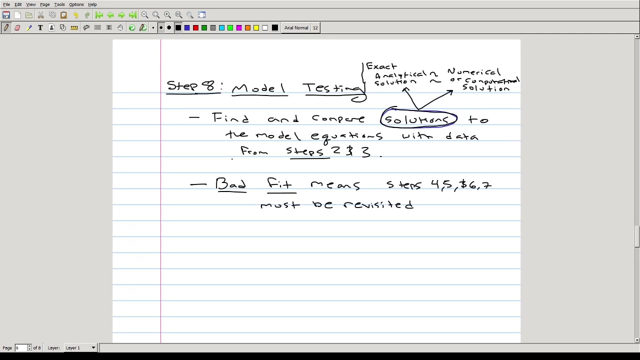 and it's at this step where- if i in this you know, testing you have a bad fit, let's say you have a bad fit to your model- means steps four, five and six and seven must be revisited Once you have a working model and you're sufficiently sure that you've done step eight here tested. 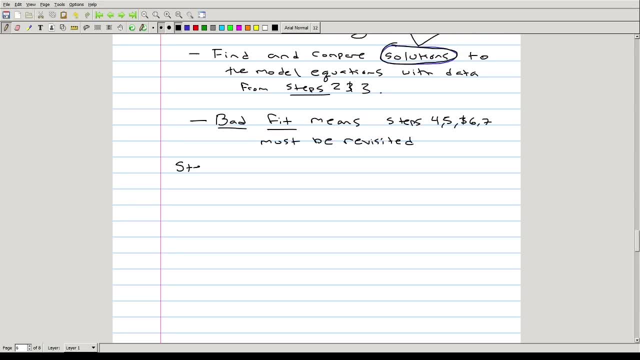 your model. Step nine Is an investigation of your model limitations and constraints in the model. So you really push it to the extreme and you figure out what the limitations and constraints of your model are. I guess all I'll say is: investigate Your model limitations and constraints. 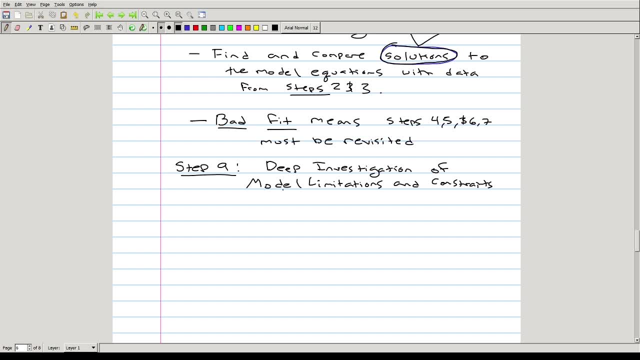 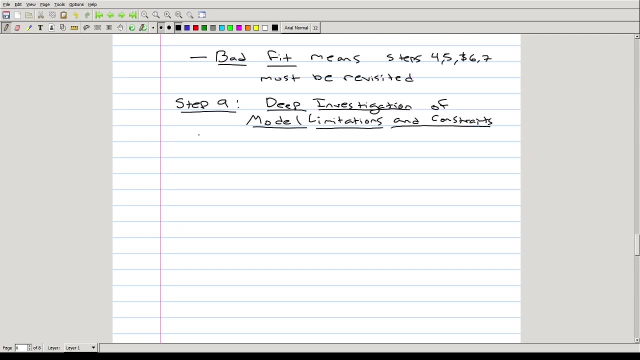 You really want to push your, your, your, your model to it's bound, its limits and the boundaries of of the model, the limits, to really test and figure out what the true limitations and constraints of the model are, Just like what we saw in the previous example. All of these steps you 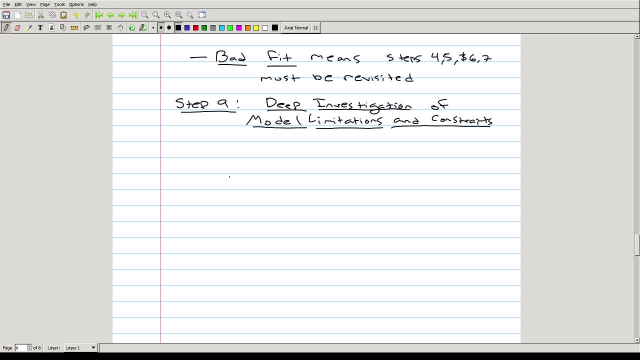 can apply to the comparison between relativity and Newtonian mechanics, but, for example, Newtonian mechanics can definitely not be used to predict motion close to the speed of light. So let's take a look at this example. Another good example that I'm going to take a look at is this: I'm going to take a look at this. I'm going to 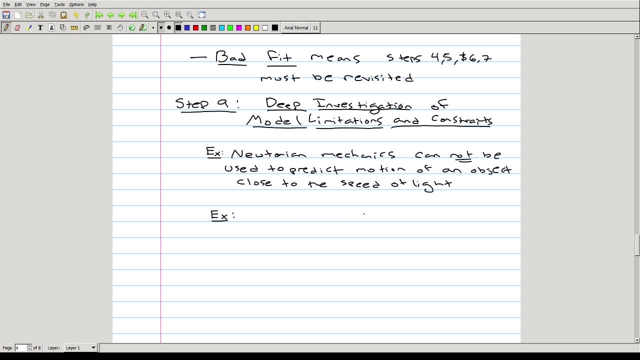 revisit a little bit later on, is the ideal gas law, which you will hopefully be familiar with from from high school or from a chemistry course. if you're taking a chemistry course, Remember this. says: Pivner P: pressure times, volume of a gas is equal to N. 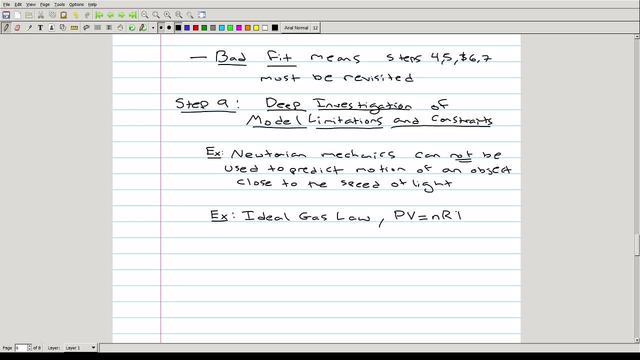 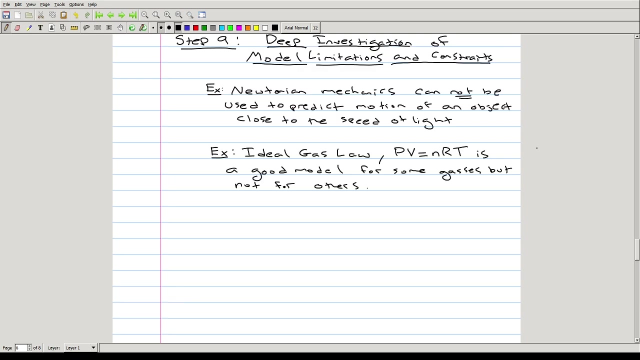 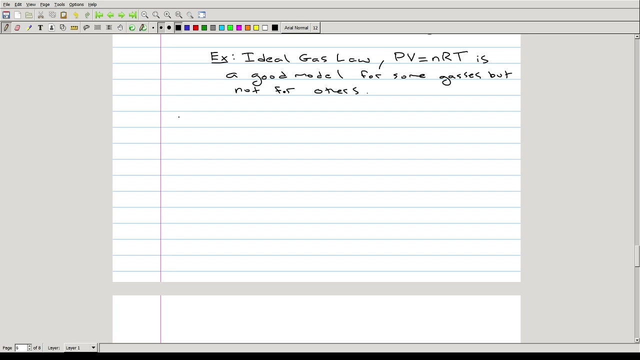 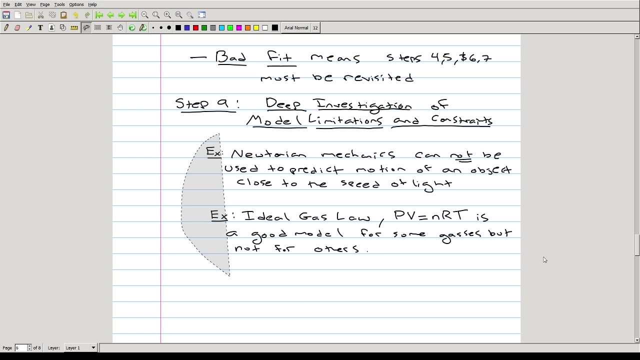 times R, which is the constant times. the temperature of the gas is a good model for some gases, but not for others. 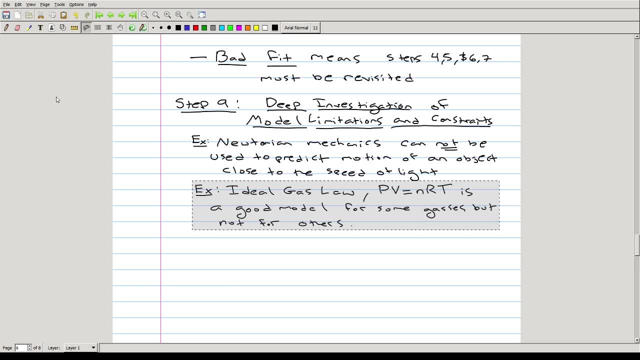 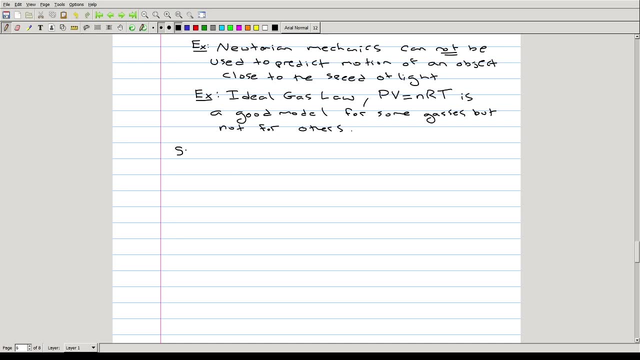 can then move on to the next step, which is what's called predictions and sensitivity analysis, and this could consist of a lot of different things, but then the main idea here is: how sensitive is the model to small variations in parameters or terms in the model. I will say variations, say in parameters. 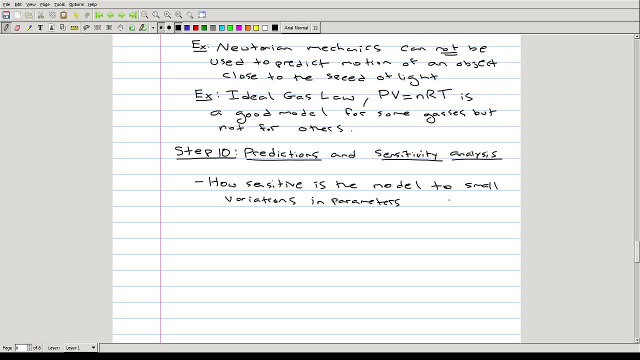 some models are required to be more sensitive than others and some less, and I'll give a good example of this here. we call a chaotic system a system that displays the following, and we'll investigate in this course a number of different so-called chaotic systems: when the evolution 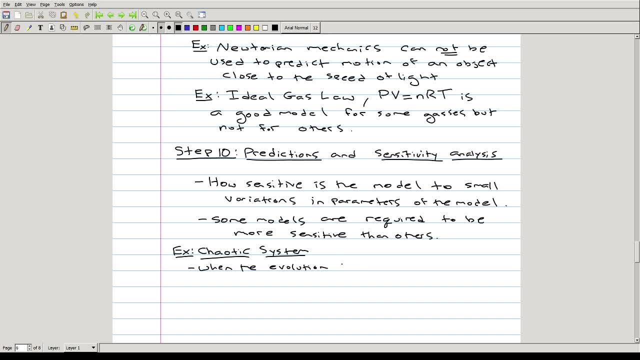 of a system displays high sensitivity and it's rather alone, first off, since there's no water in it. and this system加油, Io radio duty mission prcka. And for such systems it's only possible to make short time predictions. They're small parameters, so short time predictions are only possible. 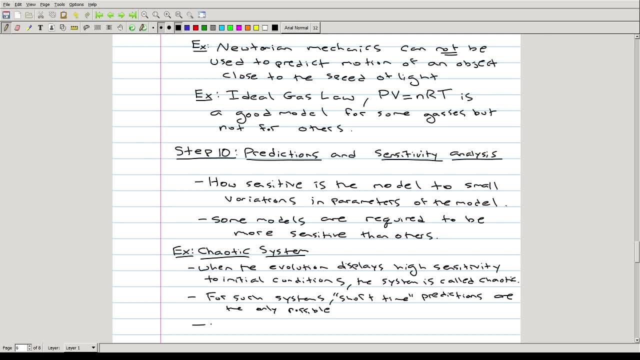 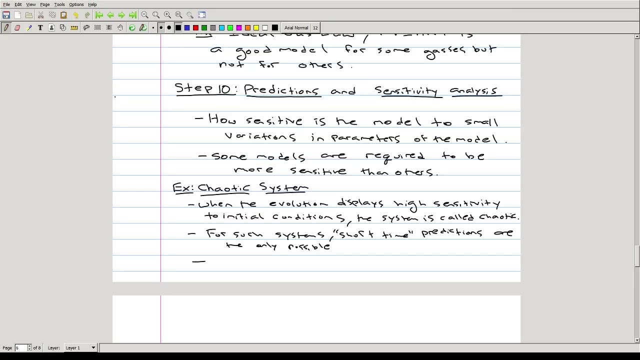 And this is a good example of why weather forecasts are accurate only for a few days- The chaotic nature of the system and that all of the variables that are going together, even a basic model for weather patterns and for the weather exhibits chaos And sometimes not at all. sometimes you get a weather forecast and the weather forecast. 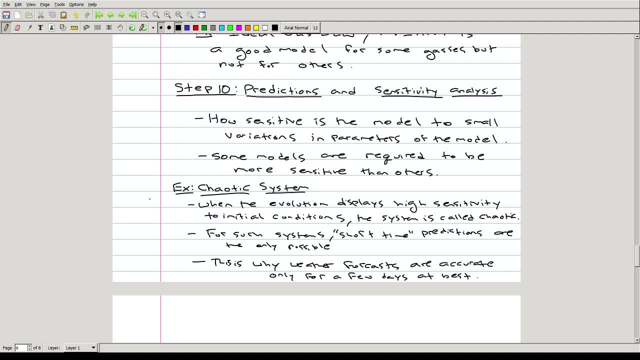 is completely different than what was predicted, So it's very, very important to see this. This is a very good example of such a system, and we'll see some system differential equations that actually come From you know basic assumptions about the atmosphere. 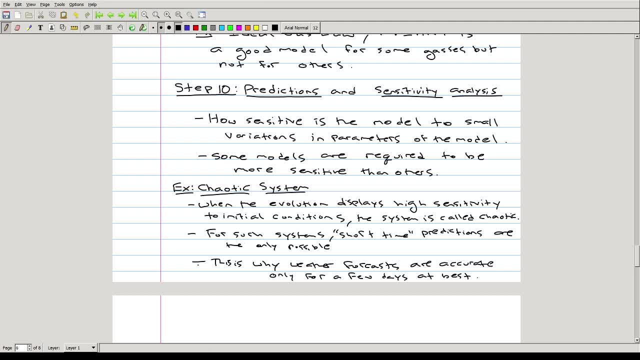 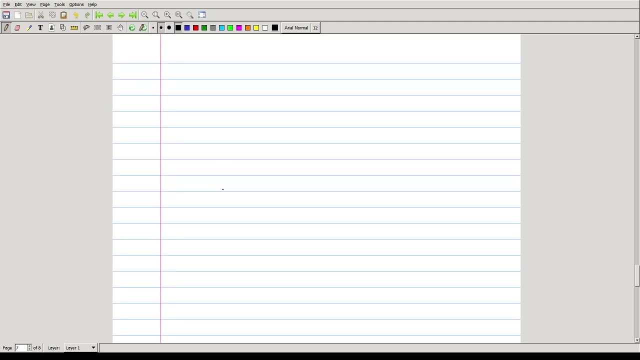 So the Lorentz equations, the Lorentz system is a fantastic example of the chaotic system and we'll actually investigate this numerically by the end of the course and see how we can approach this and learn from this. So once we've established results about the sensitivity of our system, 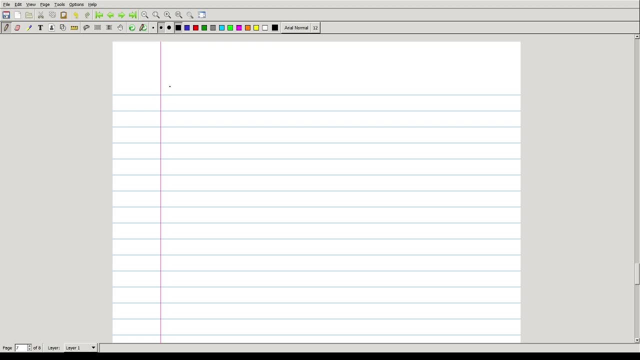 We can move on to step 11. Which consists of making extensions and refinements to the theory that we've built up from the ground, And This really consists of going back to the limitations and seeing how we can kind of update and make our theory better and more accurate to cover the things that we found. 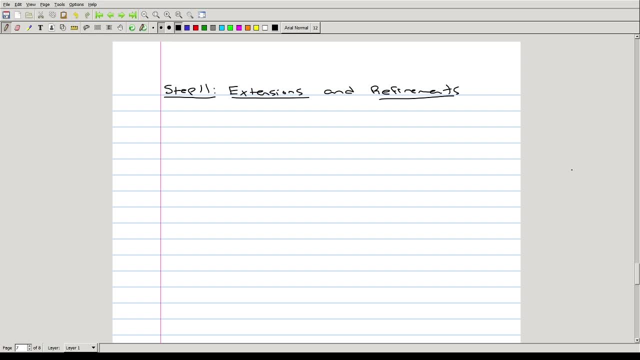 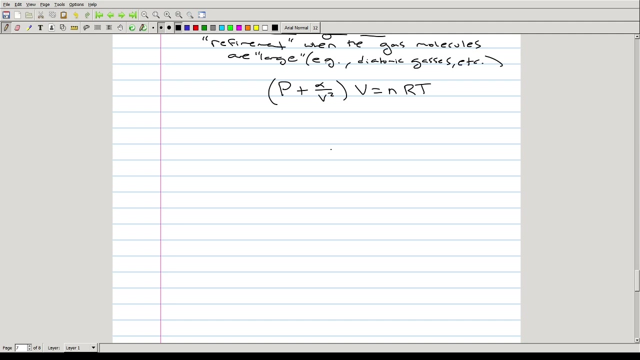 that were limitations in the previous steps. So, for example, a great example of this that I told you earlier that I would mention is that The gas law needs a refinement under certain scenarios, and they're very common scenarios. The idea here is that, under varying circumstances, the ideal gas law is not enough, and it's not. 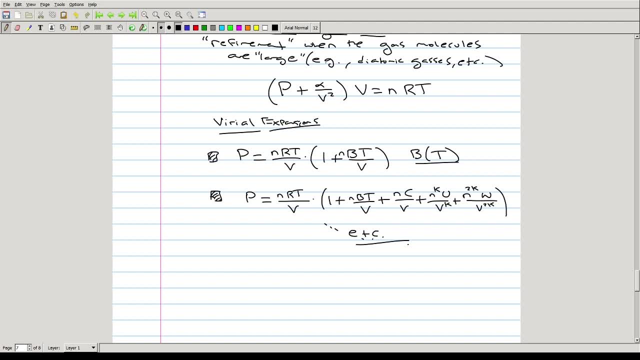 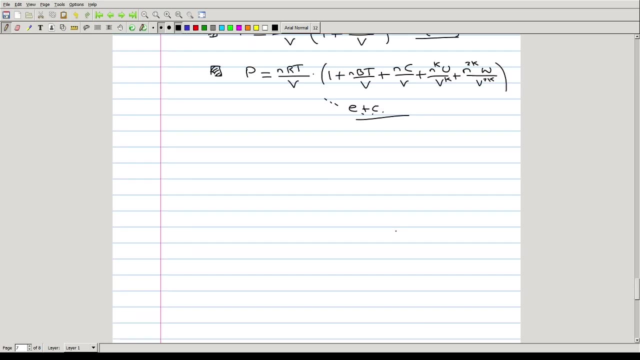 accurate at all. These extensions are more accurate and are in a refinement of our original theory. And so once we've done this, or we think we've successfully done this, You know, extended our theory and refined our theory enough, We can do what's called compounding. 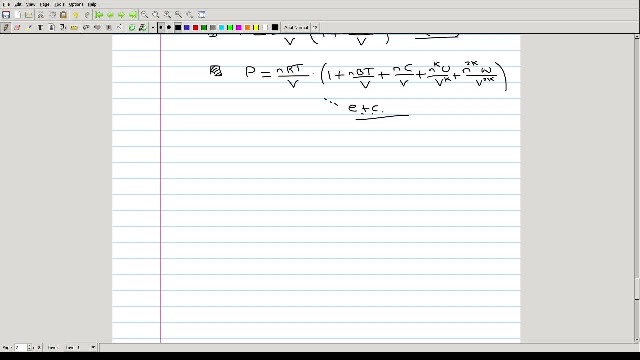 And this is the last step of this process. So once we've refined and extended our theory as far as we need it or as far as it can go, So once we have a reliable model that we found that we're okay with, we can model related. 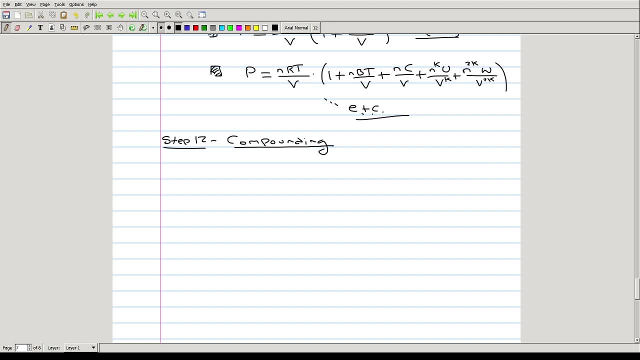 and more complex problems by compounding. And that's really what compounding is. It's kind of taking our model and building it up and applying it to larger problems And applying it to larger and larger systems. So, for example, one of the things that we'll talk about a lot in this course are both linear. 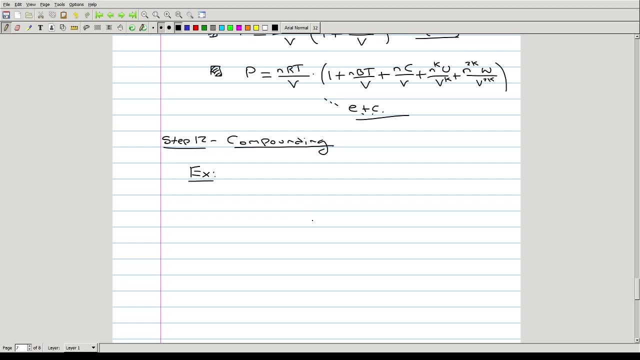 and non-linear springs. but let's just say you know. if you're, you've taken a course in ordinary differential equations or physics. you're familiar with the spring mass system. So compounding would be. you know there's steps one through 11.. 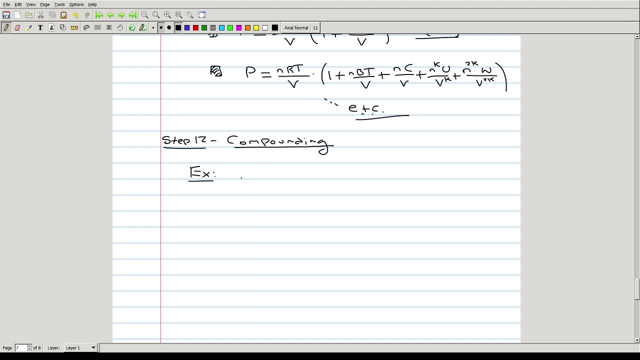 Let's say we go through and we develop a suitable model for our spring mass system. This describes the motion of a mass M and spring of spring of a mass. Okay, It's k in its motion about its equilibrium point. back and forth, back and forth, back and forth. 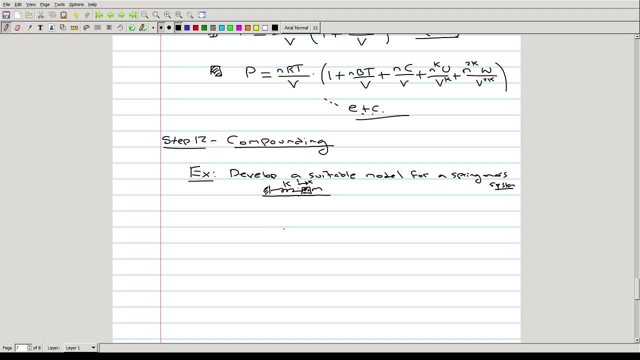 So, once we have this successful model, which you should hopefully be familiar with, we can then compound it by considering the motion of a number of different springs and masses that are connected to one another, The motion of which will be much more complicated: K1, M1, K2, M2, K3, M3, K4, M4, K5, M5, K6, M6, and so on and so forth. 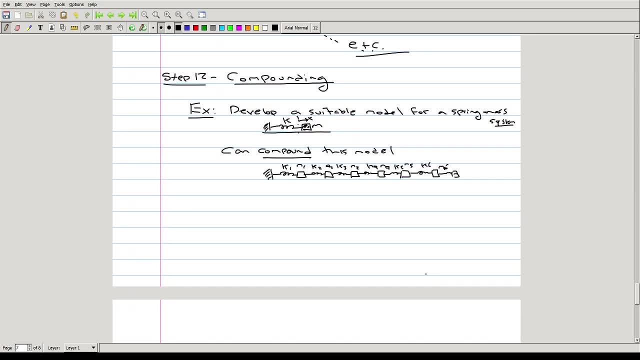 This model can then be compounded even further and used to study one-dimensional longitudinal wave propagation. This is a very simple way to do it: Along an elastic bar. Take this picture right here, This picture, Consider, you know, we continue going with it indefinitely. 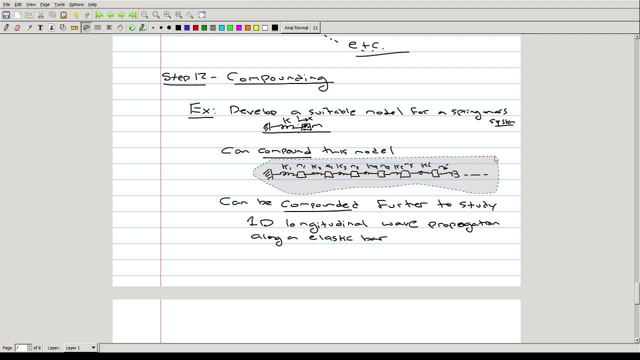 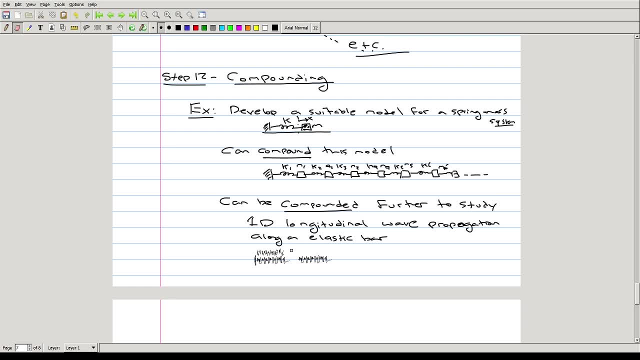 And I'll get rid of these as well. What else will this stuff be? It's going to stay at some particular place for a number of seconds. You've got to bottom up out of your way Or out of breath at that minute. 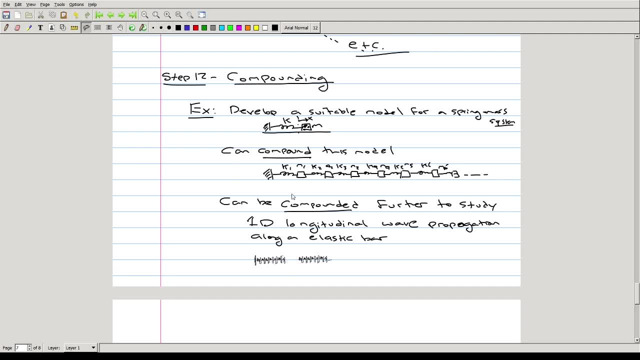 But it's new. but I know now there's so much. I've already made changes in here. Now the thing that should have stayed still is going to start back up. But we're going to go with this, Just relocate the sort which is very, very, very, very small. 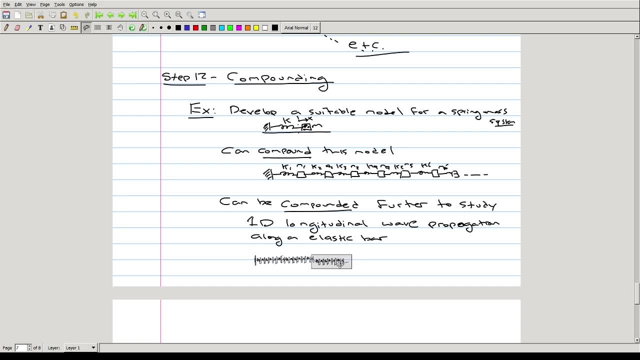 I can just pop this out. This is going to come back right at this point Because I just know, and so in the limit as this system goes, smaller and smaller and smaller and smaller. this is identical to what's called one dimensional wave propagation along. 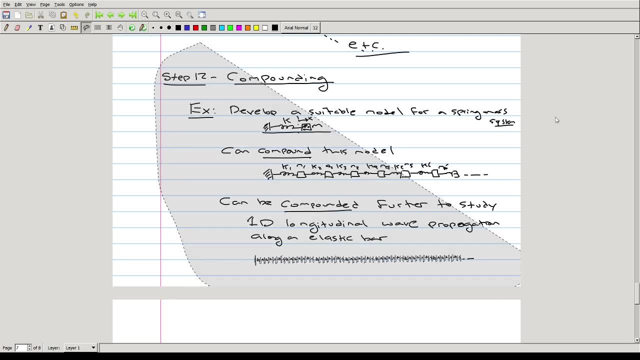 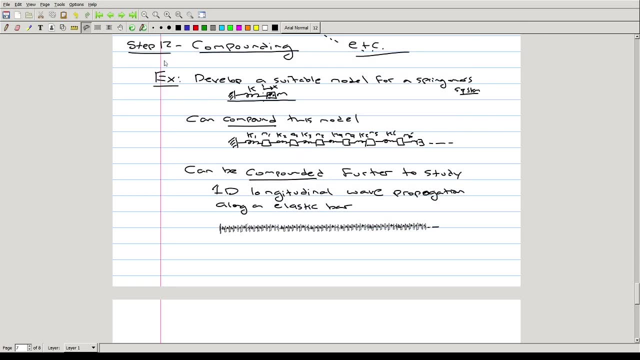 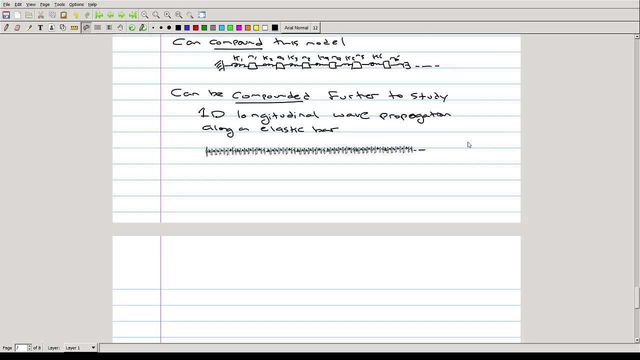 a longitudinal elastic bar. so we can show very, very clearly and concisely that the phenomena that's being modeled by this spring mass system is the same phenomena as if you have an elastic bar and a continuous elastic bar and you study the disturbances that propagate through this elastic bar. 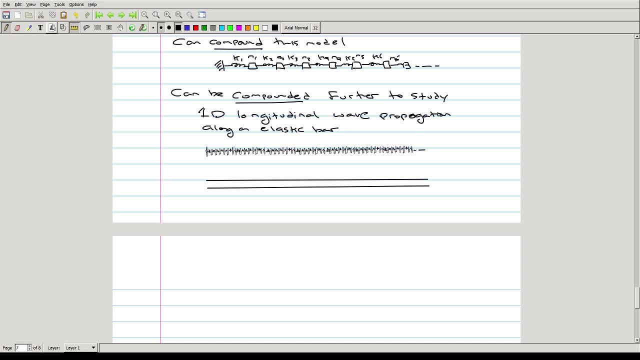 so you can say: have an elastic disturbance because you hit one end of the bar and you wanna study how this disturbance or how this wave travels through the bar. it's a longitudinal P wave. you have a P wave moving like this and a P wave moving like that. 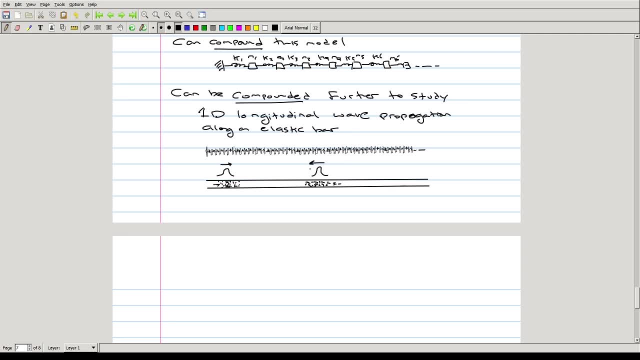 but the idea is that by compounding the spring mass model we can jump up even further to event as a series, then moving on this popular p wave by the spirit matrix, so that by quatre terminal p and the mass model now run, the Wisir is about tens Growing Lovingimbion. So that's a elite power. 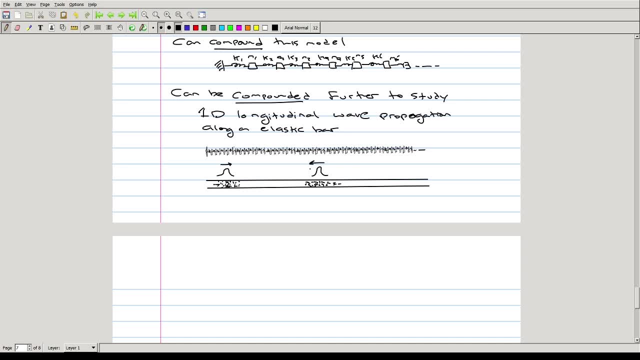 so thank God so much for listening to this theory speech learning. We leave this Click to the coco, as always. So I just wanna check out some more important information for you. if you have whatever you'd like to share, actually go from a system. So we'll see that this is a single, ordinary differential equation for the 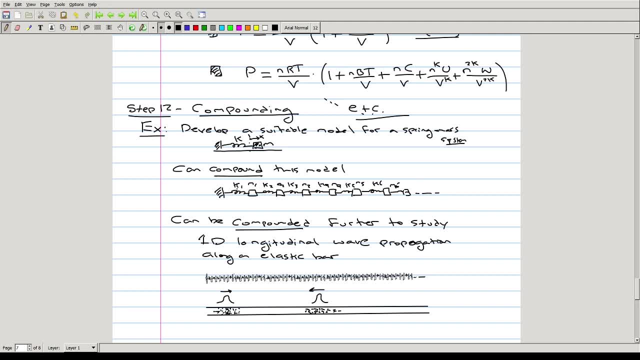 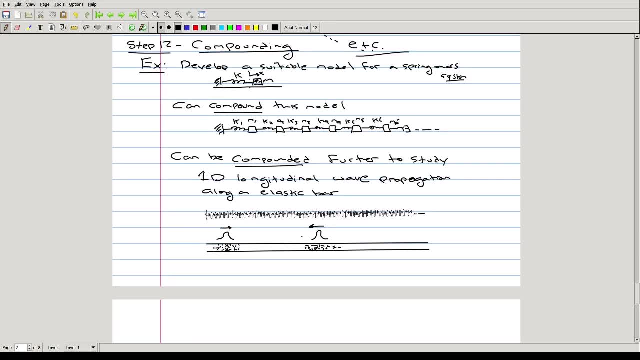 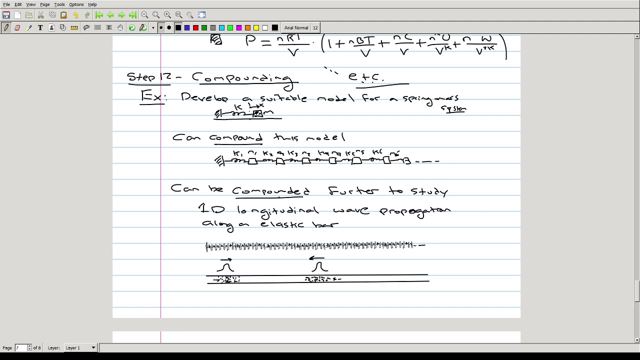 motion of this mass. This model consists of a system of ordinary differential equations that govern the motion of all of these masses And then, in the limit, we actually get a partial differential equation, called the wave equation, that governs wave disturbances moving along this bar. This is a great example of compounding a problem, And if you're wondering what a 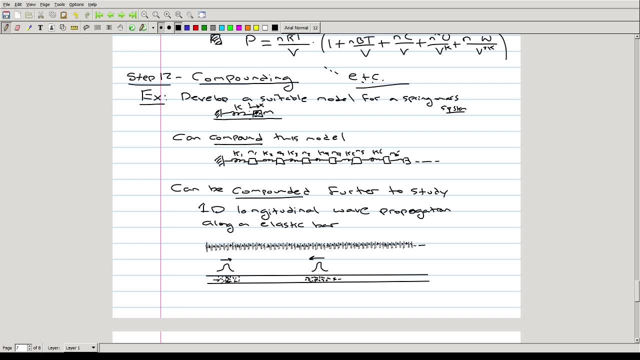 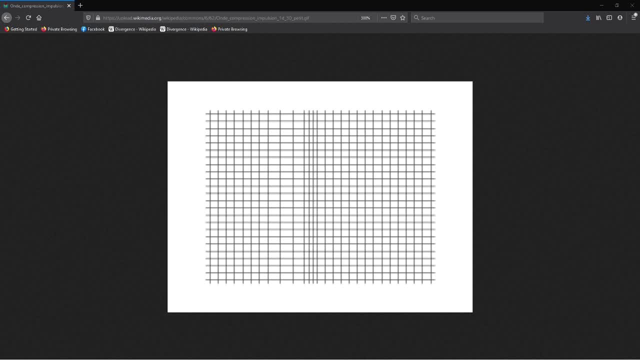 longitudinal wave looks like. I have a little animation that I can show you, So this is what a P wave would look like, or a longitudinal P wave would look like as it travels through the material, And this is exactly the behavior that you would expect from a system of springs and masses. if you 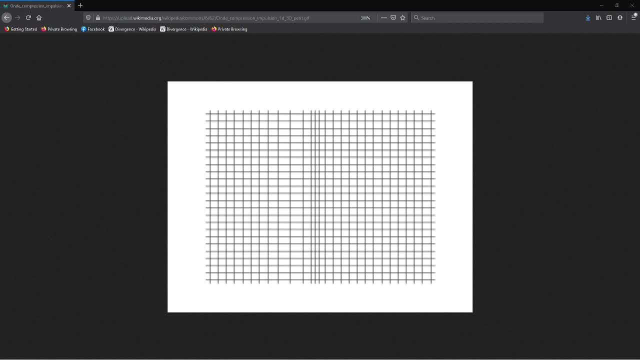 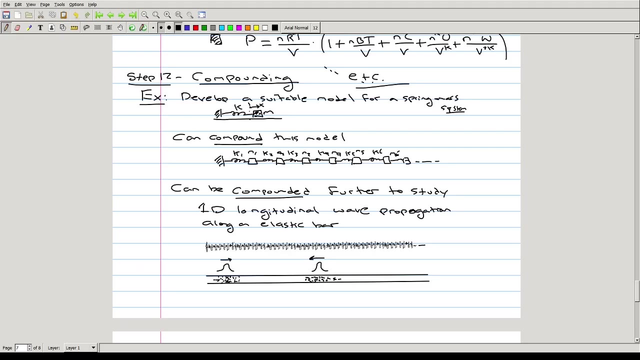 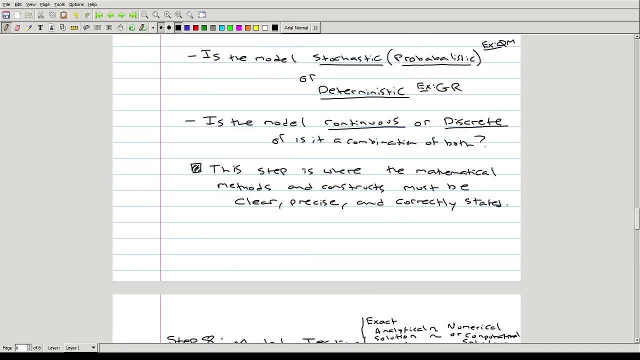 say: Jostle one end, this disturbance will move through it. So this finishes this 12 step process. essentially gives us a great summary of everything we need to know about mathematical modeling. It may at first seem a little bit overwhelming. Steps one through. 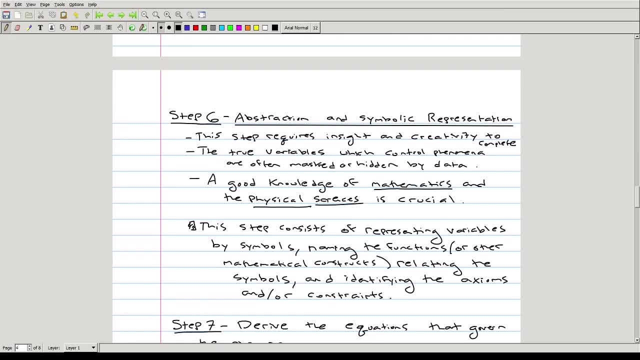 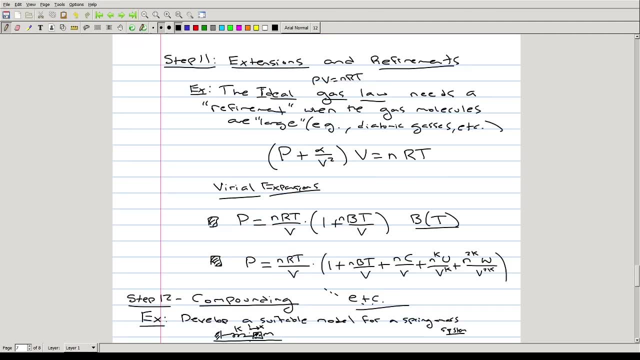 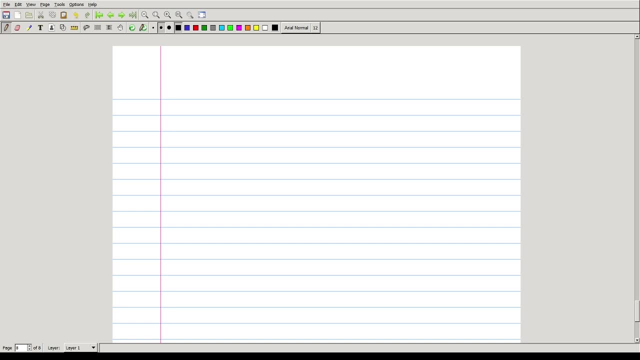 five, it's a qualitative model And in this course we'll be really focusing on step six through 12, which is, you know more, computing a quantitative model or finding a quantitative model of a phenomenon. And again, I can't recommend Meyer-Humey's book enough, so much so that he does a 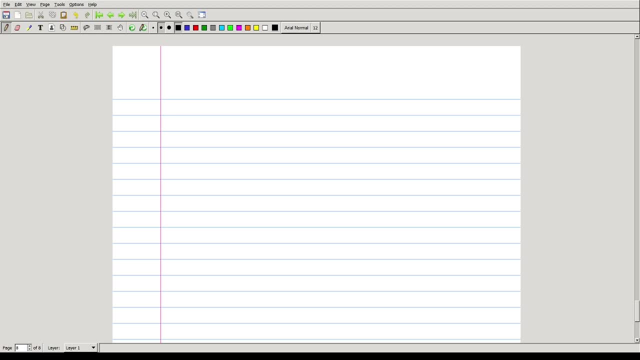 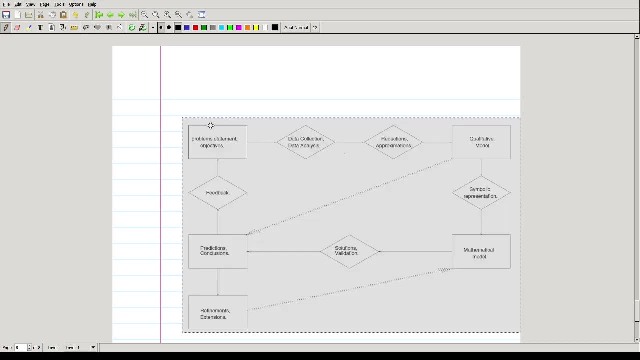 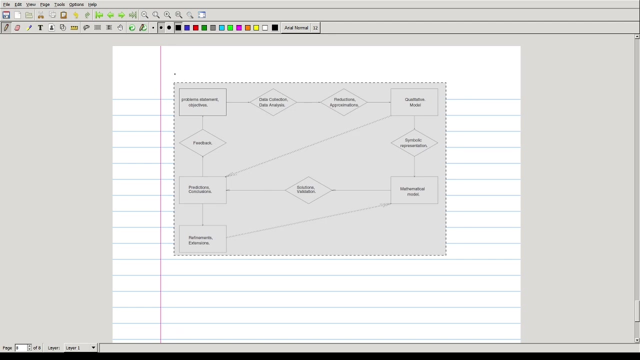 great kind of like summary in this chapter. Uh, in the Qiührer's book, it lists all the results that went through, And then it says everything that I'm interested in. So it's- this is also everyone's daily notes, a short summary of them, a wonderful knowledge source that will now include in these.